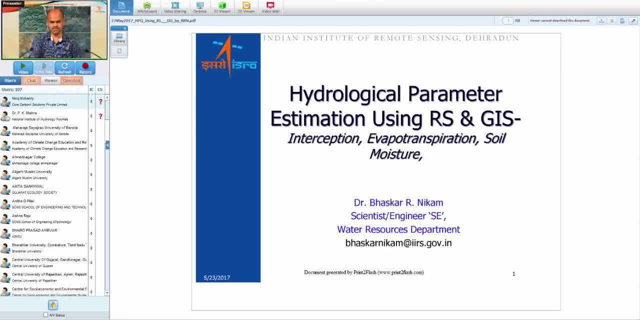 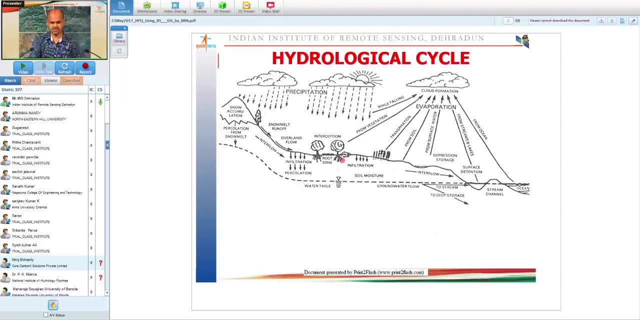 So I'll be talking how we can use remote sensing as well as GIS, which is a handling tool for remote sensing data for estimation of interception, evaporation and soil moisture. So, if we just want to touch the basics, we know the hydrological process is a cyclic process, So if we receive rainfall, it will be infiltrated in a soil, which will be stored in the soil as a soil moisture. 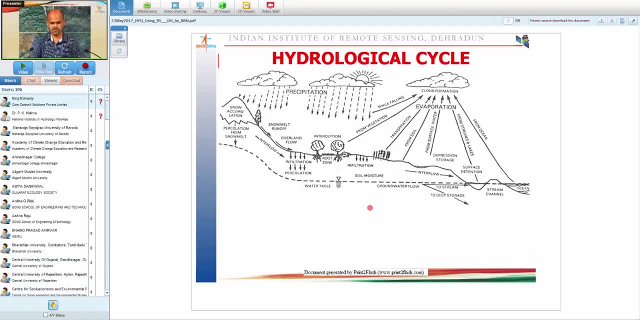 The excess water will flow over a surface as a runoff. then it will be stored in a local distribution, So it will flow through rivers and join ocean. From the every surface having water, it will be evaporated again, join atmosphere While the rain is happening. not the entire water will touch down to the surface. 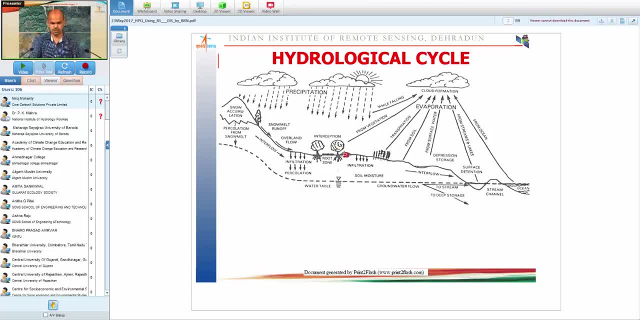 The upper story, which could be your vegetation or could be the dead leaves which you call litter, will intercept some of that water. So if we are in, if your purpose is to estimate actual hydrological components at every state, we need to consider all these. 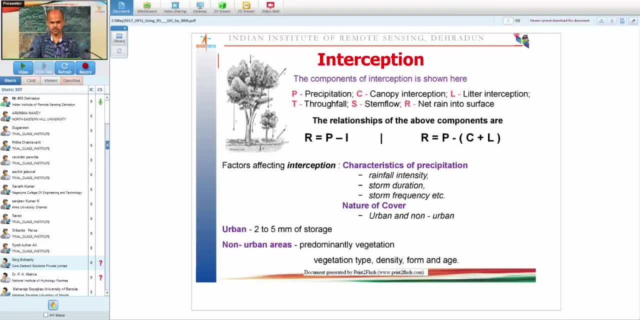 Part of all response乐 This: these aspects of hydrological cycle. So if we want to talk about interception, understand this process of interception. if pee is the rainfall that we are receiving, If it's a bare soil, the entire pee will touch down toward to the soil. 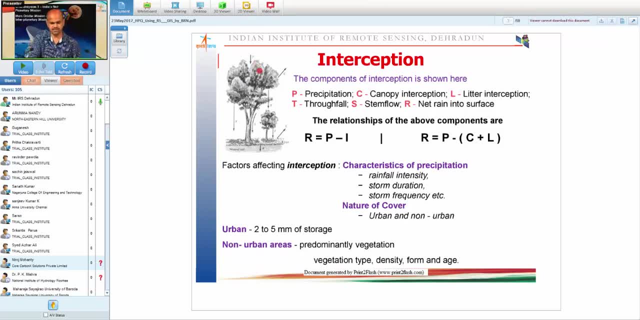 But if we have a vegetation or story on a soil, So if we want to talk, is being overfilled so that water will be released either as a through fall or it will flow as a steam flow. now, if you have a litter on ground, litter will also. 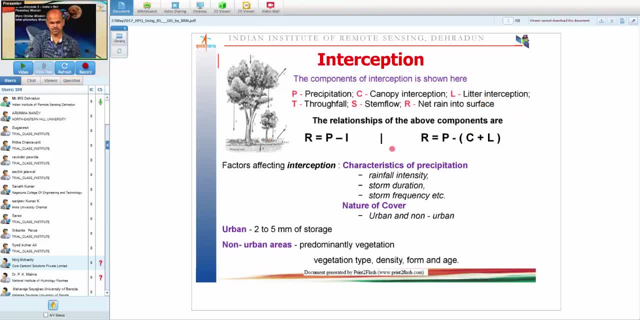 intercept some water which we term as a litter interception. so, mathematically speaking, the water, actual water that reaches to soil for infiltration, is precipitation minus interception. and if you want to divide interception into two components- interception by crop or vegetation and interception by litter- so you can do it and we'll try to see how we can estimate interception using 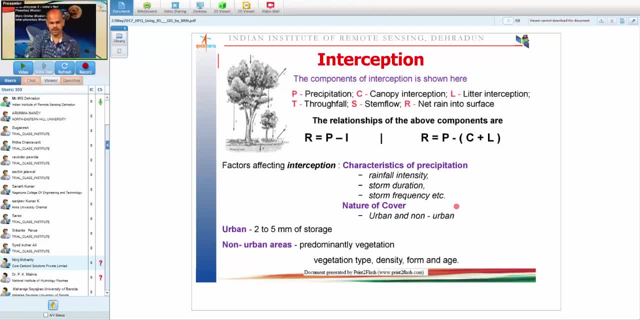 remote sensing. but basically interception depends on two main parameters. one, it depends on characteristics of precipitation, like rainfall intensity, storm duration, storm frequency, and it also depends on nature of vegetation: what kind of cover you are having. do you? do you have a bare soil? or if you have a urban cover or non-urban vegetative cover? if we have urban cover, 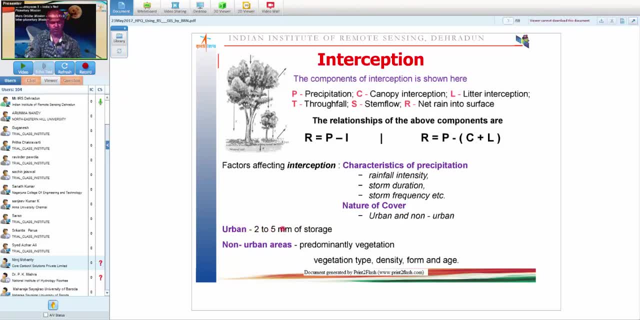 we generally use a thumb rule that around two to five mm of water will be released in the soil and then the soil will be released in the rain and the precipitation that we are receiving will be intercepted. but if it is a non-urban cover, the amount of water intercepted depends on too many. 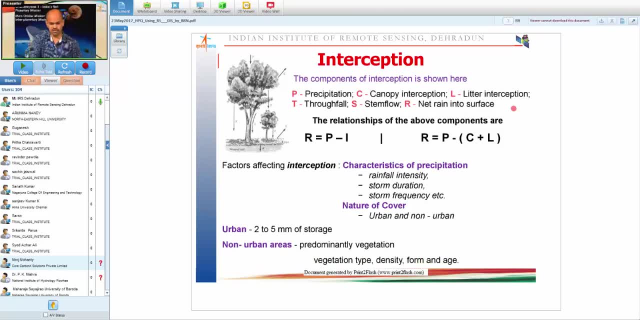 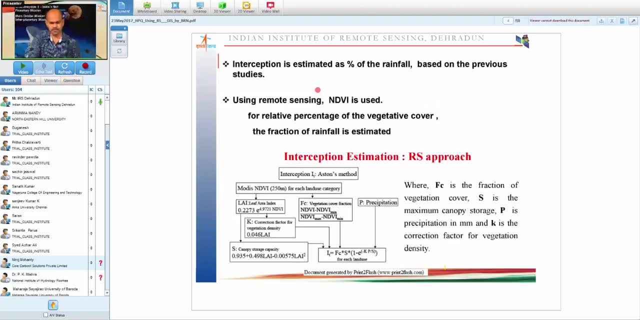 parameters like vegetation type, vegetation density, form of vegetation, age of vegetation. so generally people go with a simpler approach. they take a person, they use a land-use map and then just assign a percentage that if my land use or land cover is urban, let's say 1% of my rainfall will be intercepted. but 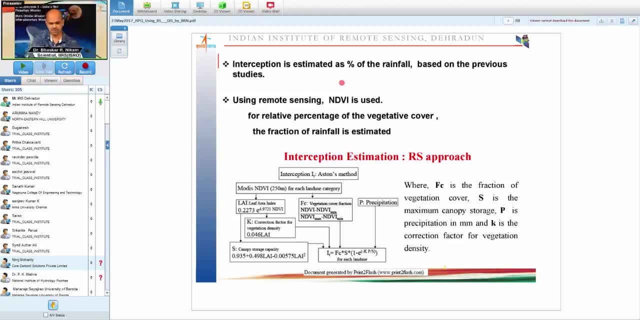 but if it is a, let's say, vegetation, other percent will be intercepted. but in case of vegetation, defining a specific percentage may not be correct because vegetation changes its state with time. crop in the month of January will have higher density than the crop in the month of November, so interception rate. 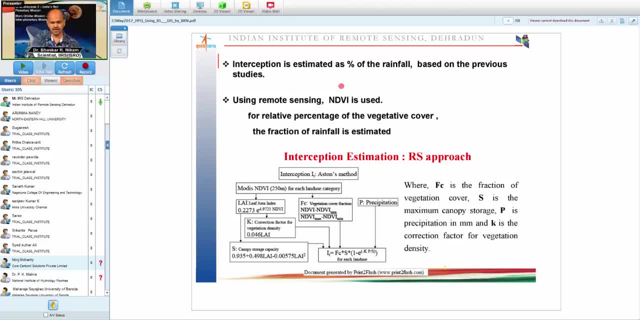 will be different, so another alternate approach could be: we can link the interception rate with vegetation and generally to represent vegetation health and density. NDVI, normalized difference, vegetation index is the parameter preferred. so we'll discuss briefly. we'll discuss one method used for interception estimation which is given by Aston's, is called Aston's method, where we use NDVI. 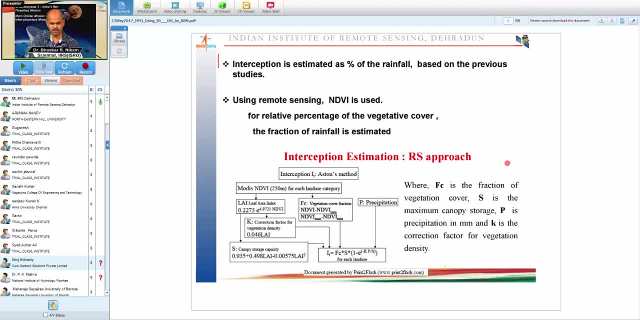 the specific method is designed or developed for modis NDVI, which is of 250 meter resolution. so from NDVI we will first calculate the leaf area index, which tells me in a 1 meter square area how much area is occupied or covered by leaf. now LAI could exceed value 1 because there are number of stories of 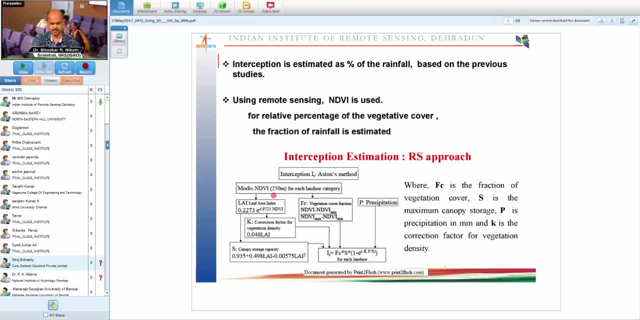 leaf. so if I only one story and the entire area is covered by leaf, LAI value will be 1, but if I have multiple story of leaf, so LAI could exceed more than 1. now, from NDVI, I will also calculate the fractional cover or within a grid. so 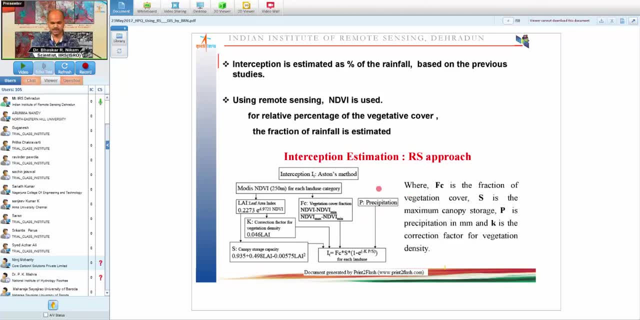 which is simply we, we make a standardized of NDVI. now I'll take a precipitation information from LAI. I will calculate the storage capacity of that canopy S. S is a storage capacity of canopy and K is a calibration constant or correction constant for different types of vegetation and its density. so once I 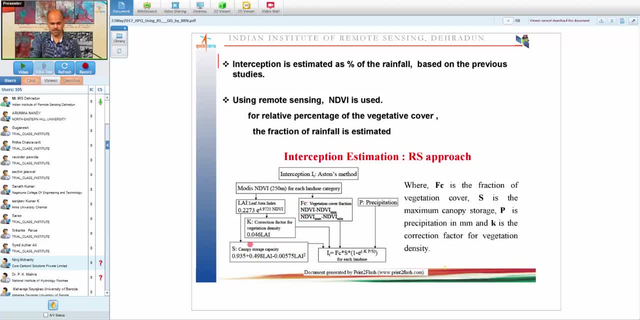 have the fractional vegetation cover, the storage capacity of that vegetation and the correction factor with precipitation, I can calculate the interception. now this is not the only method. there are many methods. people have related this interception with LAI. they have related this interception with only the fractional vegetation cover to. there are many methods used, but the point here is: 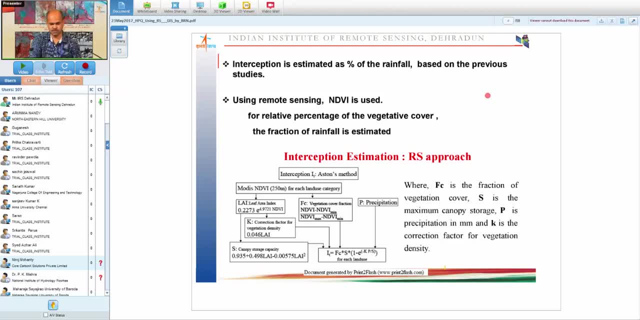 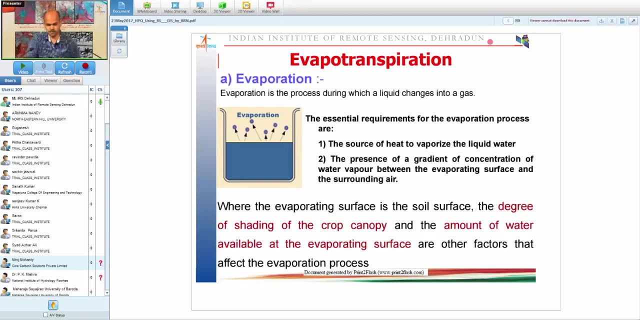 remote sensing data has a capability of giving synoptic coverage to whatever I am observing. I'm not observing for a point, I'm observing for a area and, as we know, the land cover will change with space. so this special dynamics of interception can be captured using remote sensing data. now we will touch. 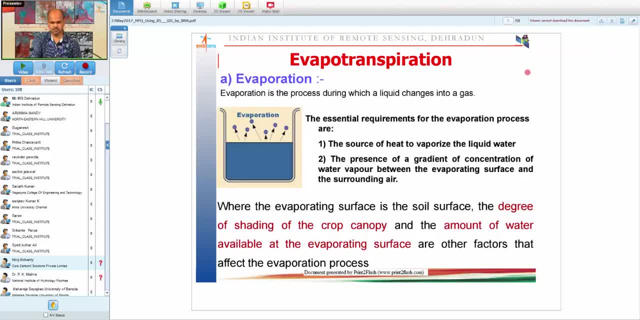 upon evapotranspiration in the hydrological cycle. in a sense of importance, evapotranspiration is the most important component from a volume balance point of view and from energy balance point of view, If we talk about any general watershed, 30 to 60% of water that a watershed receive will. 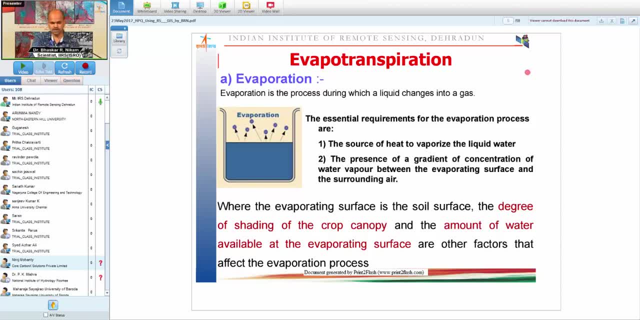 be lost or will be consumed by evapotranspiration. On the other side, out of total energy that we receive on any scale- day or annual or monthly scale- something around 77% energy that we receive from sun will be used for evapotranspiration. 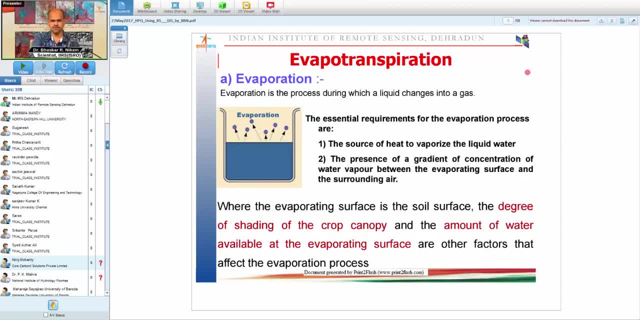 So in that sense in hydrological cycle evapotranspiration is the very important component. But evapotranspiration is a combination of evaporation plus transpiration: Evaporation through which we lose loss of water from a water free water body which requires essentially source of energy and there should be a saturation gradient between the surface. 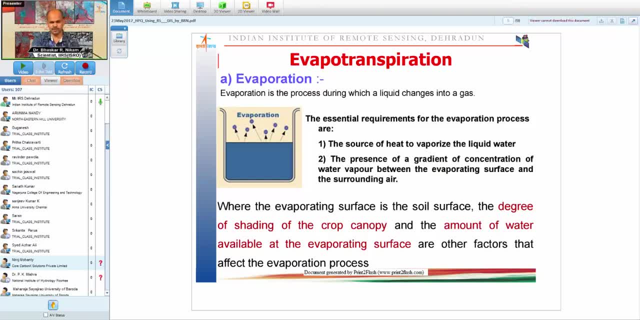 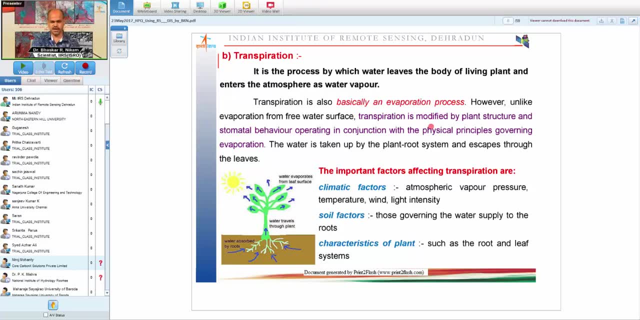 from where evaporation is happening and the medium where the evaporated water is going, Whereas the loss of water from the plant surface Is called as transpiration and as we can understand, because here the surface from where the loss of water is happening is a plant surface, 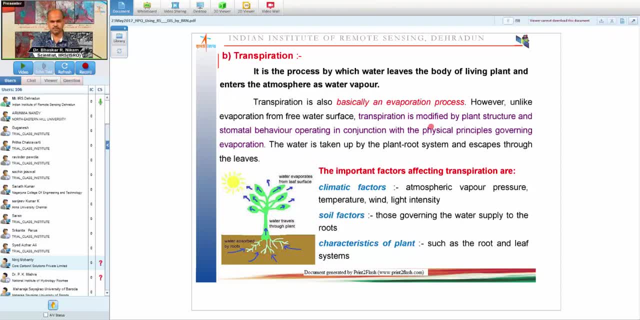 So along with all the factors that govern your evaporation rate, the biophysical parameters of plant also govern your transpiration rate. So if I have to calculate or model evaporation it is bit simpler compared to if I want to calculate or model transpiration. 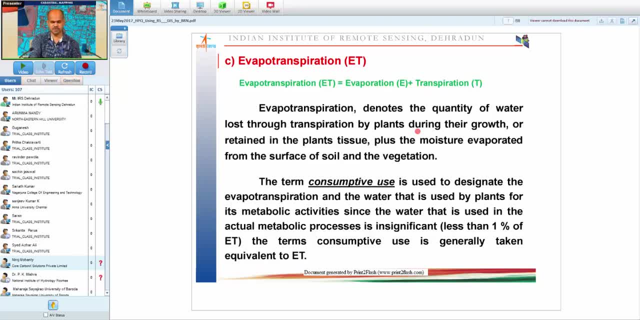 And evapotranspiration is a combination. when I say combination, it is a summation of evaporation plus transpiration. So maybe either of this will have a value and other will not. still evaporation. evapotranspiration will have a value. Why I said this? because typically for transpiration to happen we require direct solar radiation. 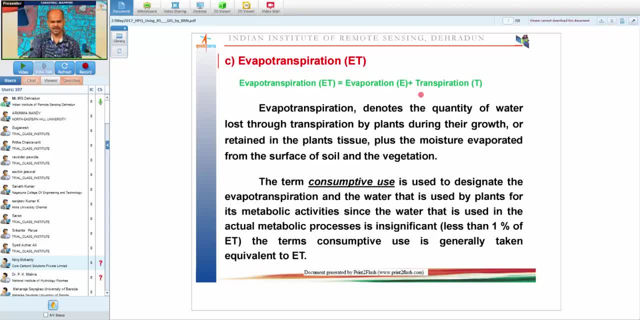 not even diffuse direct solar radiation. So we all know in the night time we don't receive direct solar radiation, short wave radiation. So in night time transpiration will be zero. But for evaporation to happen we only require source of energy, which we do have in night. 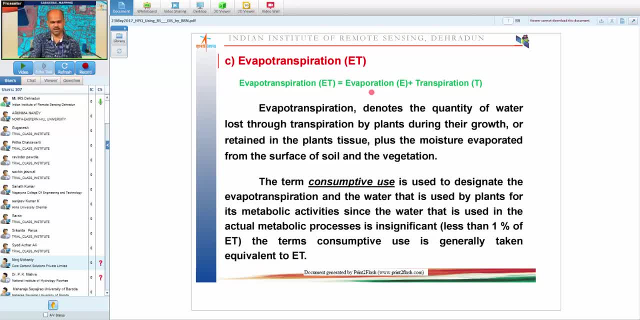 time and saturation gradient between the surface from where evaporation is happening, which will be a water body or a soil surface, and the medium where that water is leaving, which is a air. So there will be a saturation gradient. So as long as these two things are there, evaporation will happen and so evapotranspiration will. 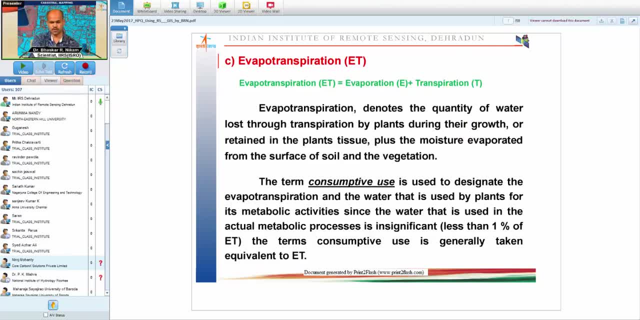 happen, though the transpiration is not there. Now, when we talk about in sense of irrigation or agriculture, we also have a term called consumptive use. So consumptive use is nothing, but if we calculate evapotranspiration, Add 1% over that, which we assume that the water- this means water- will be used by the. 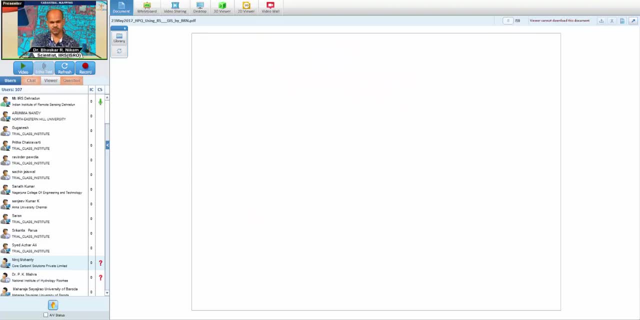 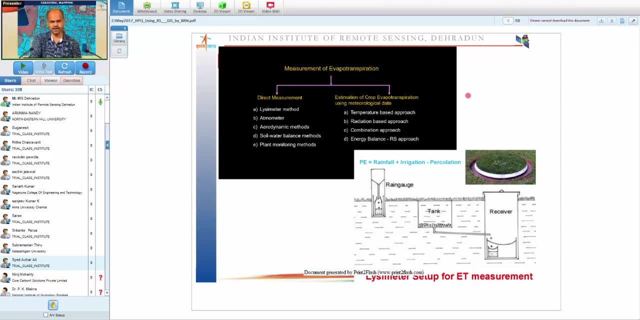 vegetation for completing its metabolic activity, and that total we call it as a consumptive use. Now, since evapotranspiration is very important process, we should have instruments to measure it, as well as we should have methods to calculate or model it. So, based on the data used for calculating evapotranspiration, we basically classify the 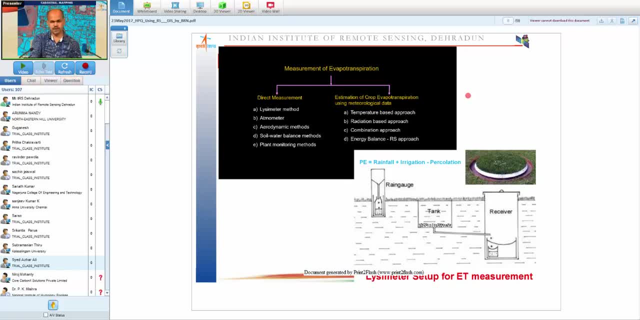 methods used for evapotranspiration. For example, if we use temperature data for calculating evapotranspiration, we call them temperature based approach. If we use temperature plus radiation based data, we call them as a radiation based method. If we use temperature radiation plus some other biophysical data, we call them as combination. 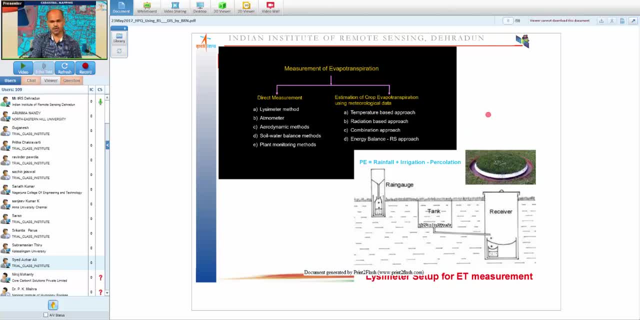 method and the last one, which is a recent one, if we use remote sensing inputs for calculating evapotranspiration, we call them remote sensing based energy balance approach for calculation of evapotranspiration. So that is what we are now using. In the bottom of the slide I am trying to show you apparatus which is called lysimeter. 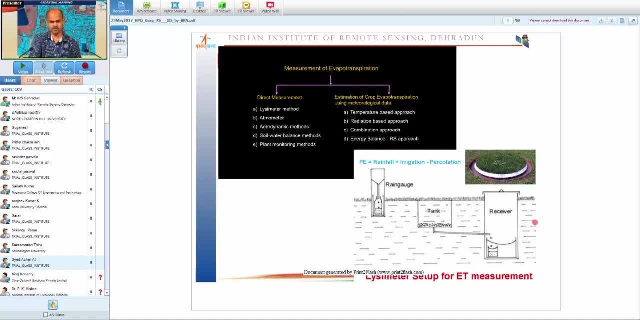 which is generally used as a reference apparatus or reference instrument for calculating or monitoring evapotranspiration. Please note we are not monitoring evaporation from this apparatus. We are monitoring evapotranspiration: Transpiration from the crop or plants grown in this apparatus, plus evaporation from the 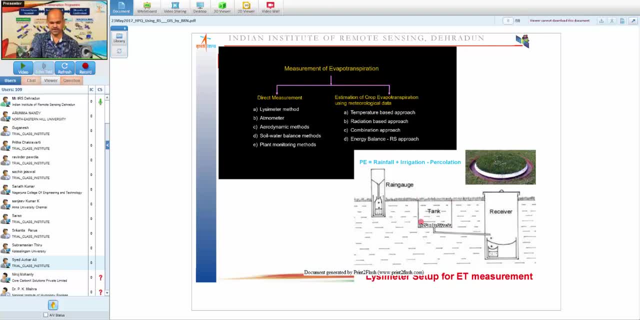 soils, which is there, And, as you can see, the soil is isolated by a metal cylinder, because of which there will be no lateral water movement. So whatever water we will have here will either pass through vertically downwards, which we can collect and measure, or it will loss vertically upward, which we call evapotranspiration. 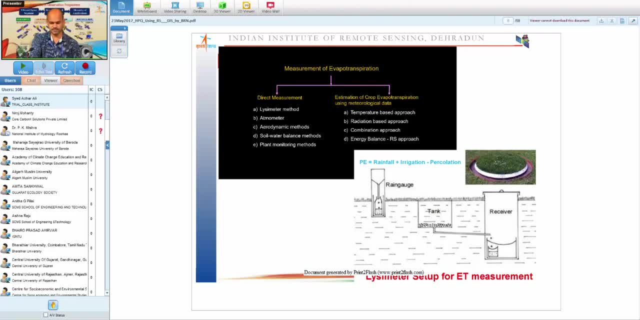 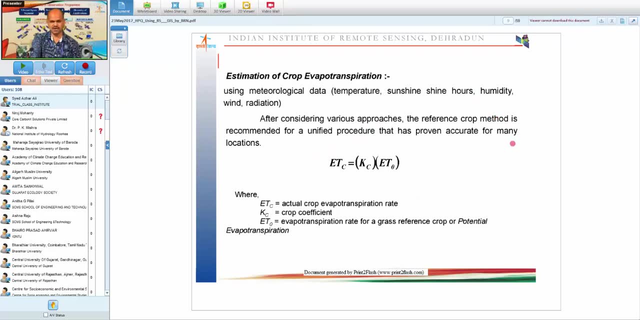 So this basically works on the principle of volume balance or mass balance. The observations for lysimeter are used as a reference observation for calibration and validation of any newly derived evapotranspiration method. Now, since evapotranspiration, Transpiration is a combination of evaporation and transpiration and, as we all know, transpiration 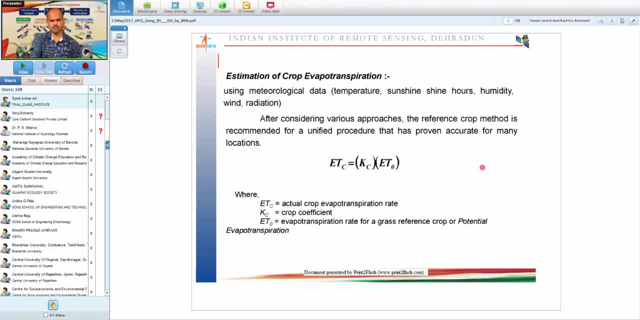 is governed by biophysical parameters of vegetation. Biophysical parameters of vegetation will vary with time and space, So it becomes very difficult to model it, because the data required for modeling or estimation of evapotranspiration is simply non-existent. So practically what we have done 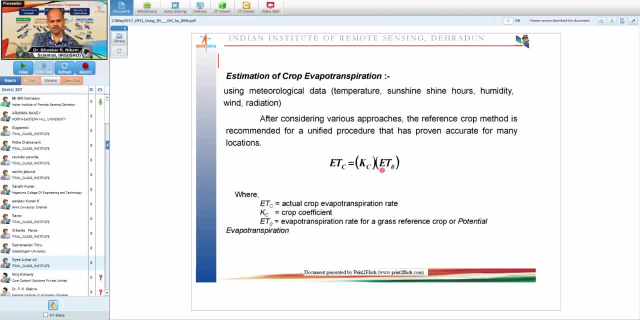 We have divided evapotranspiration into two terms, wherein the one term represents evapotranspiration, which is a potential of air to cause evapotranspiration, which we call reference evapotranspiration, and another term, which we call crop coefficient, represents the impact of the surface, like 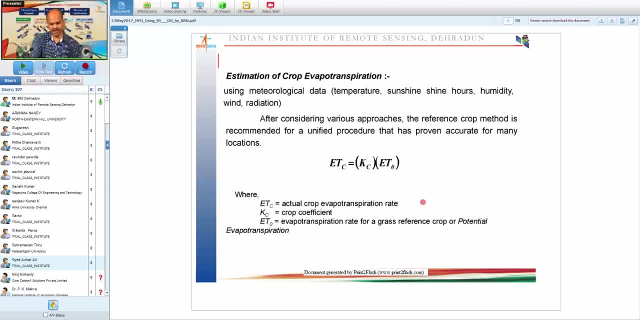 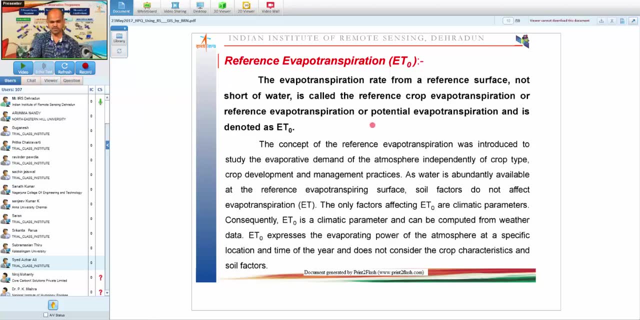 biophysical parameter and availability of water in soil. on the actual evapotranspiration rate, We will see in coming slides. So reference evapotranspiration is a evapotranspiration rate from a reference surface, as the name itself indicates And because it is evapotranspiration from a reference surface. 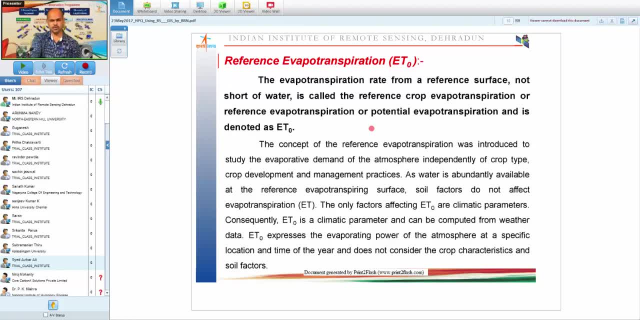 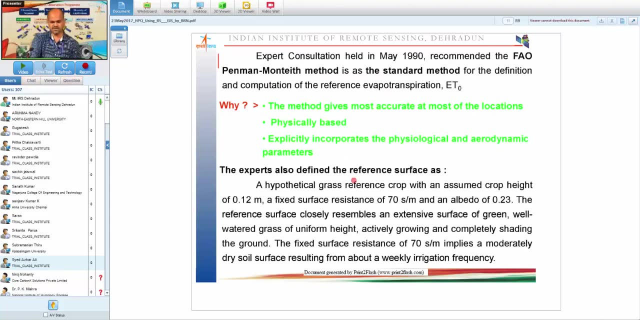 For which I have defined the reference surface. The impact of crop parameters or vegetation parameters and soil parameters on evapotranspiration is being nullified. So this reference evapotranspiration is a potential of meteorological observations only Now. the expert consultation held in 1990, have designated FAO Penman-Montith method. 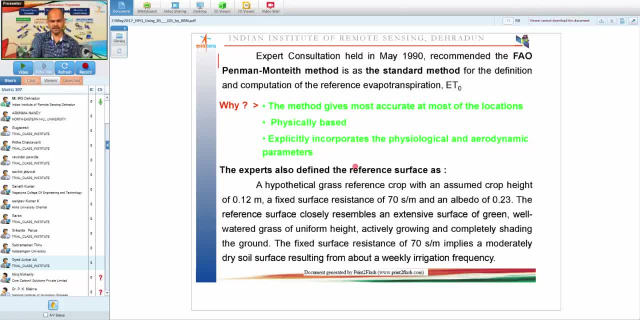 alternately known as modified Penman-Montith method, as a standard method for estimation of reference evapotranspiration. Why? Because this method gives highly accurate results in all the locations on the globe. This is a physically based method and this explicitly defines the physiological and aerodynamic 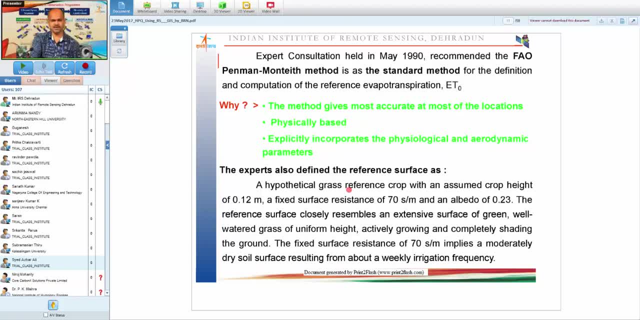 parameters involved in evapotranspiration. Now, in previous slide we said this method gives us evapotranspiration from reference surface. So the definition of reference surface has to be very specific and precise. So we define reference surface as a hypothetical grass reference crop. 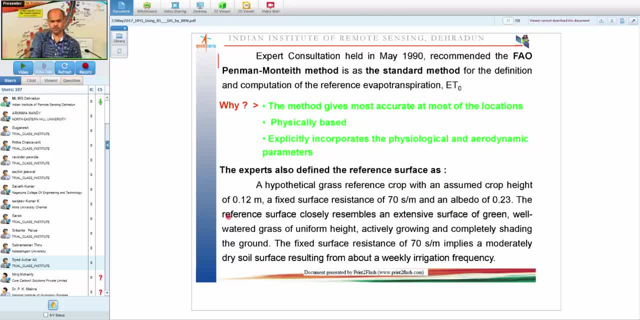 This is having hypothetical grass crop having assumed height of 12 centimeter or 0.12 meter, having fixed surface resistance and having fixed surface albedo of 0.23.. This reference surface also closely resembles to an extensive surface with green well watered. 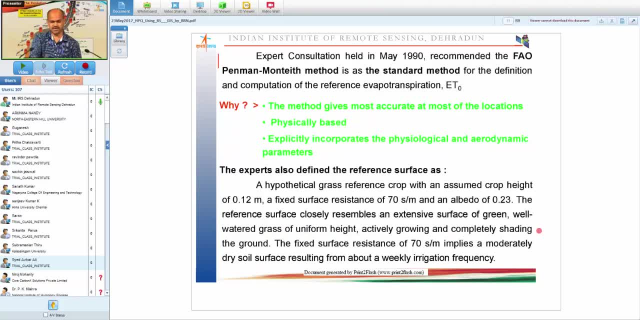 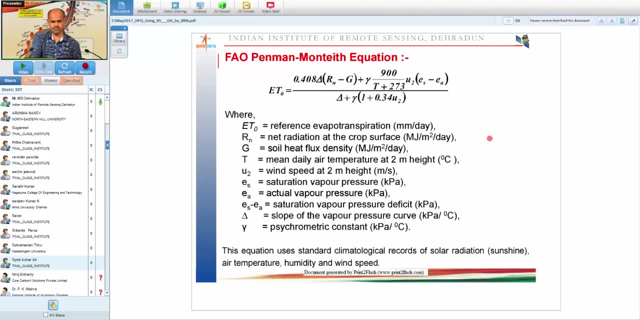 grass of uniform height actively growing, completely shedding the ground and the fixed surface resistance shows the soil moisture status. What is the soil moisture status Which is not at field level capacity? it's little bit dry, which resembles the weekly irrigation frequency. Now the reference. 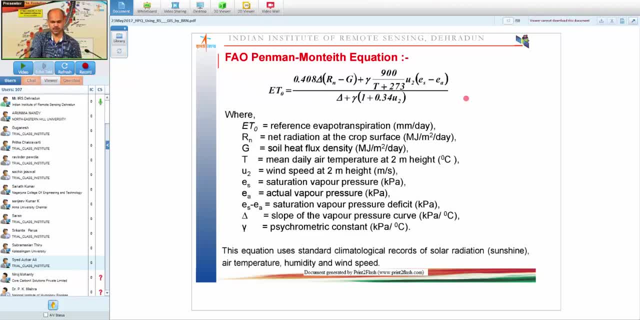 method which we generally follow is Penman-Montith method, as you can see on your screen. This method requires observation of daily solar radiation or hourly solar radiation, then your ground heat flux, atmospheric temperature, humidity and wind speed. If you have these observations, you can estimate. 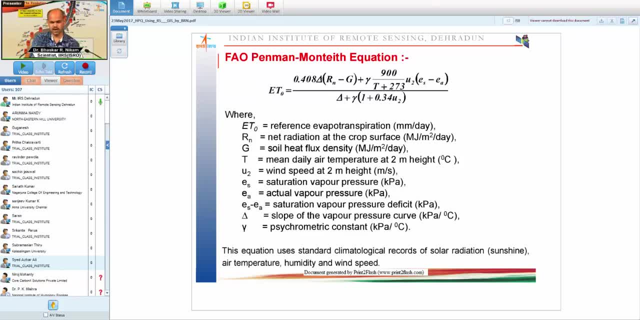 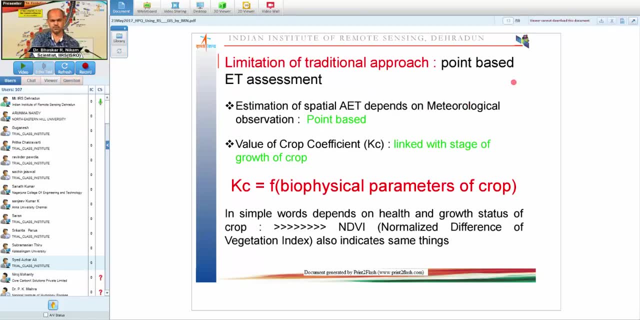 the reference evapotranspiration for daily time step or hourly time step. But the problem here is because reference evapotranspiration can be estimated using only the metallurgical data and that metallurgical data will necessarily be from a point. We cannot employ number of observatories, metallurgical observatories, to our entire. 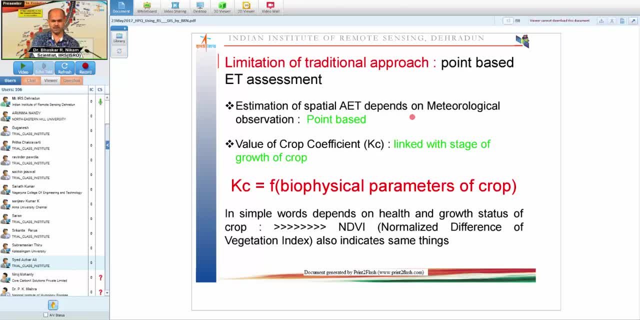 watershed or entire area. You can represent area by 1 by 1 meter pixel or 100 by 100 meter pixel. In any case, you won't have, or you will not have, metallurgical observatory representing every pixel. and other problem with the traditional approach is the crop coefficient, which is other part, which is the second. 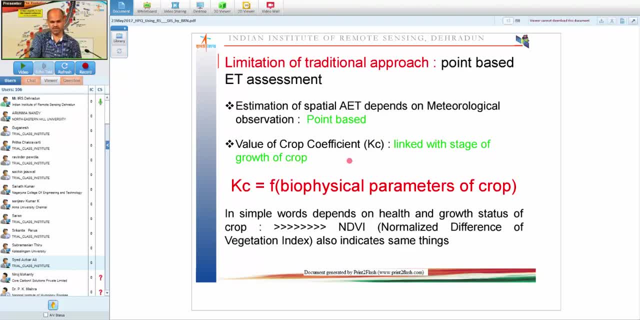 part of your actual evapotranspiration is linked to crop growth stage. So I don't know if the crop I am representing is actually at that growth stage. This growth stage is linked to the time of sowing and the time from sowing. So in traditional approach I am limited to a point observation and I don't know. 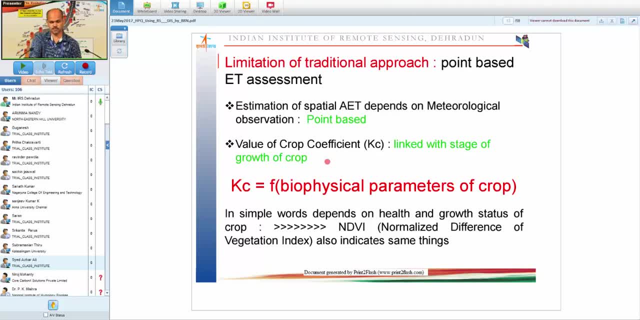 for the area I am calculating whether my crop is at that stage or not. But the advantageous part in this Casey concept is crop coefficient is a function of biophysical parameters of crop, So it could be density of crop, health of crop, the growth stage of crop And if you remember the basics of remote 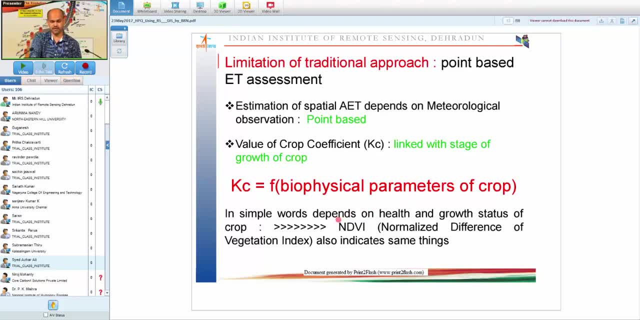 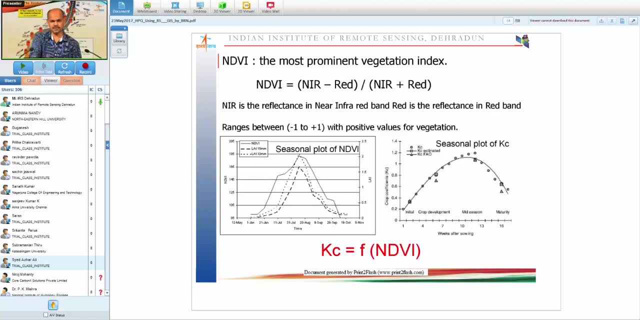 sensing. all these parameters are represented very well by the index called normalized difference vegetation index. So this gives us opportunity to correlate this normalized difference vegetation index with crop coefficient. So, if we can see on this slide, the first graph represents a typical plot of normalized difference vegetation index and LAI for a particular 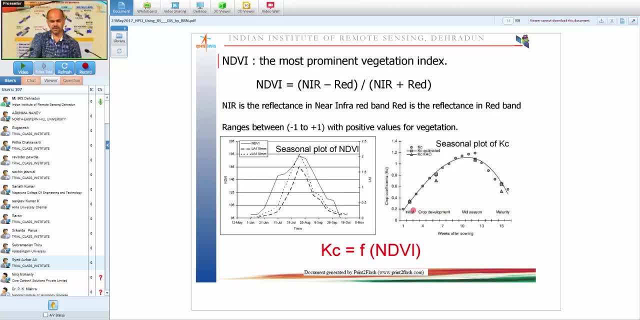 crop, which is a wheat crop, and the second graph represent the crop coefficient values for the season for the same crop. So, as you can see the nature of, if you ignore the local deviations, the nature of graph is almost same. And if I have two graphs they may differ in their numerical values but if their nature is same I can say with the confidence that there will be a relation between these two graphs and most probably that relation would be a linear relation. 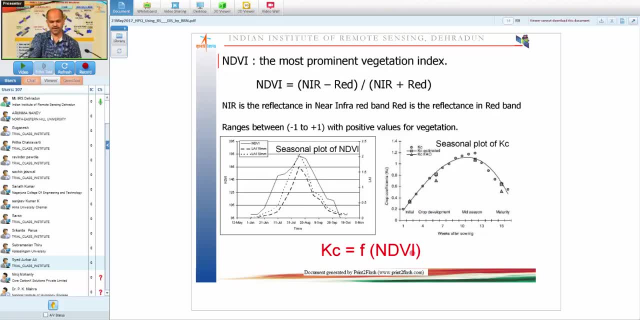 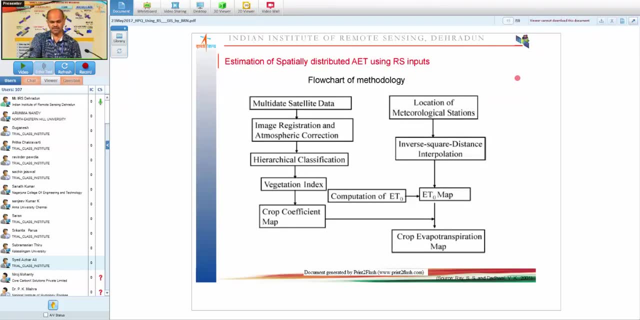 So we are assuming that there will be the Kc will be function of NDVI, because NDVI represent all the parameters on which Kc depends. So I will try to show you a approach used by many researchers to use remote sensing data to overcome the limitation of point based evapotranspiration estimation. 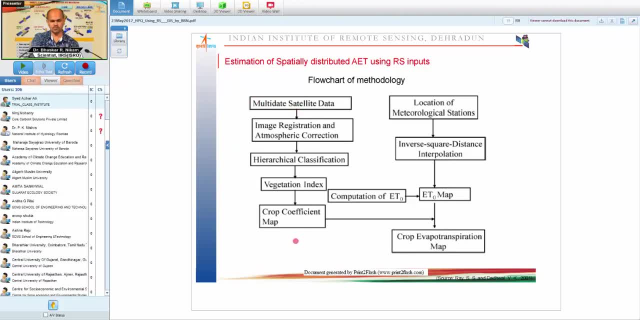 In this approach there will be two columns. in one column we will use remote sensing to calculate crop coefficient for every pixel. in other column, we will calculate the evapotranspiration reference- evapotranspiration using metallurgical observations. If I have multiple observations, I will interpolate them because I need. 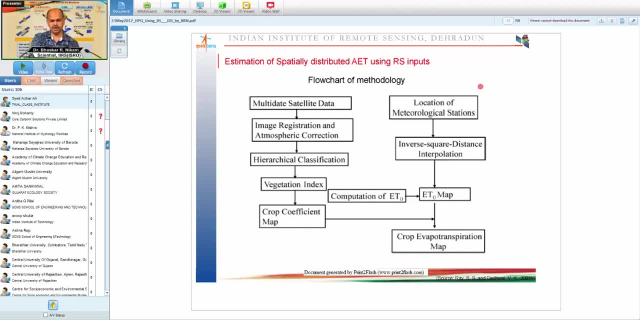 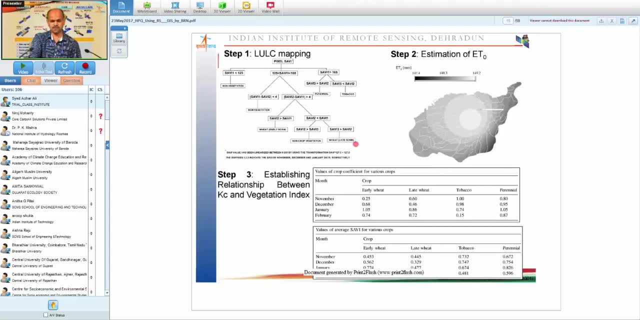 The reference evapotranspiration for all the pixels. if I don't have, I can still assume the same value for all the pixels, or I can still use interpolation approach. So here the step one would be: because crop coefficient, we are saying the Kc, will be function of NDVI and it is quite obvious that two crops, two different crops, can have same NDVI. 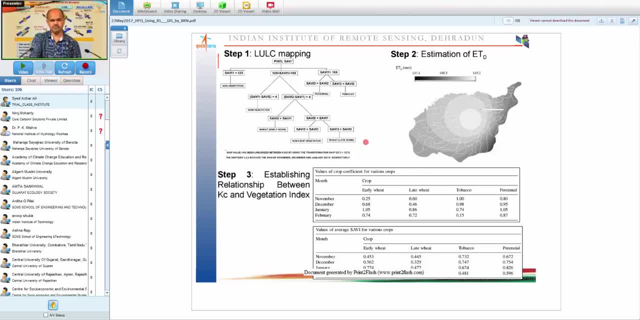 And hence, if Kc is a function of VI, I have to partition it for each and every crop or each and every vegetation type. So necessarily, my step one becomes: I need a land use, land cover map where I should discriminate between different crops or different vegetation types. 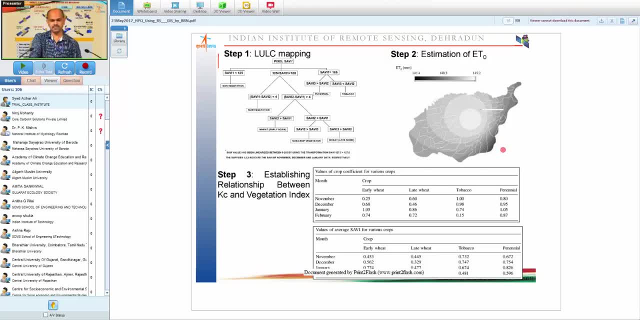 Step two would be collect a metallurgical data. based on type of data that you have, calculate the reference evapotranspiration using the suitable equation. If you have all the necessary data for applying Penman-Montith method, it is better. if you have only temperature data, you can use temperature based method. 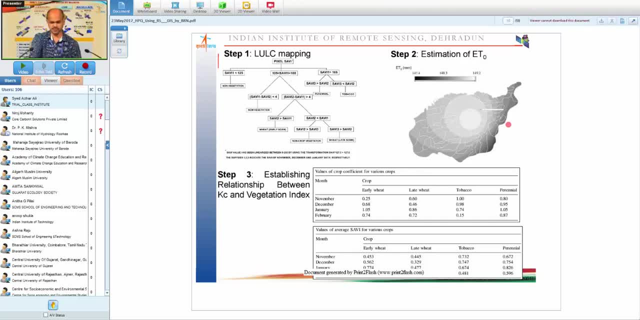 If you have radiation data, you can use temperature Or radiation based methods. Now step three would be: I will have temporal data of remote sensing. I will have temporal Kc data for those vegetation types. You can see this first table shows me, for these four vegetation types, for every month, what will be the value of Kc. 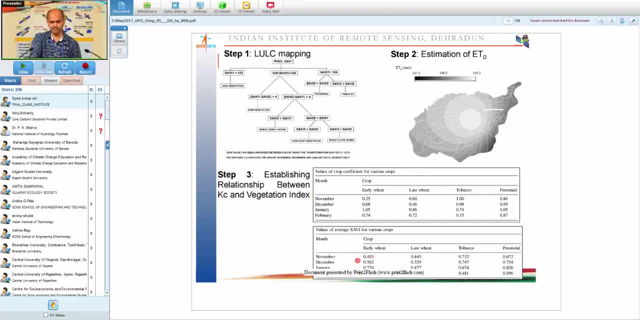 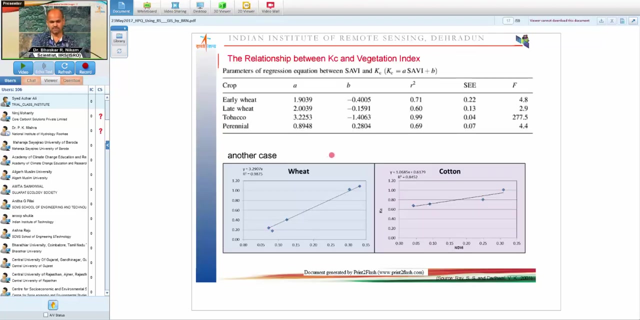 Similarly, from remote sensing data you can derive this value, value of vegetation index. in the specific we have derived the soil adjusted vegetation index. So for same months for same crop- pardon, we have derived the value of vegetation index. Now I can use these values of the specific crop in a regression equation, or I can perform a regression to get the equation of straight line. if it is a straight line, I will get a slope. I will get a slope, then intersect and these are the error parameters. 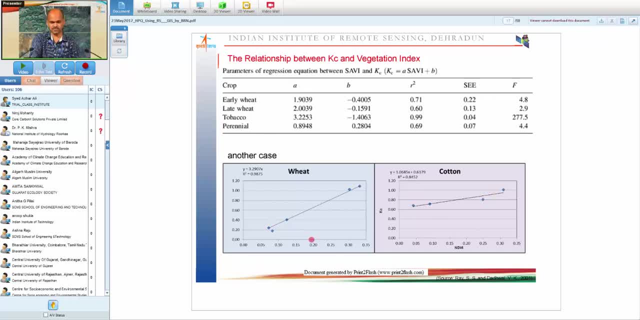 And these equations will. these lines will look like this, Where slope will be different, Intersect, And these are the error parameters And these equations will. these lines will look like this: Intersect will be different, but these lines will be that, with higher degree of confidence that I can correlate my vegetation index with Kc. 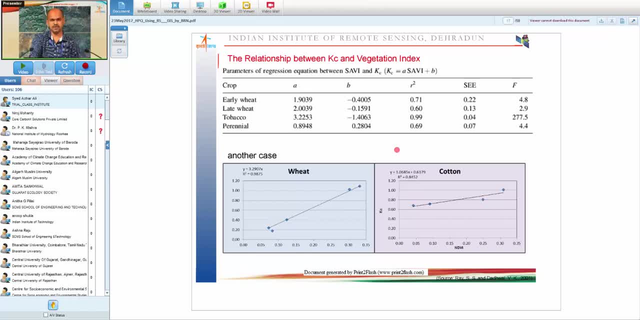 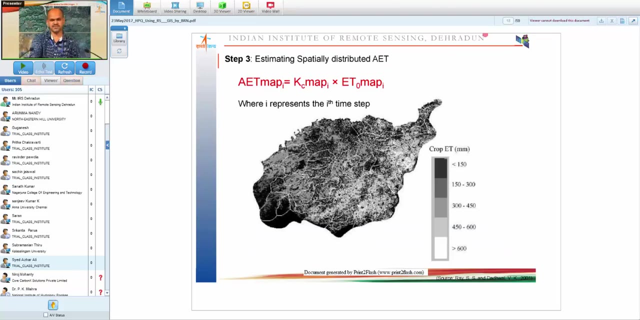 And since I can get specially distributed and temporarily varying NDVI or vegetation index, so this gives me the capacity to generate specially varying and temporarily discrete Kc values. So I may get remote sensing based on the special resolution you are interested in. if you are interested in 56 meter resolution. 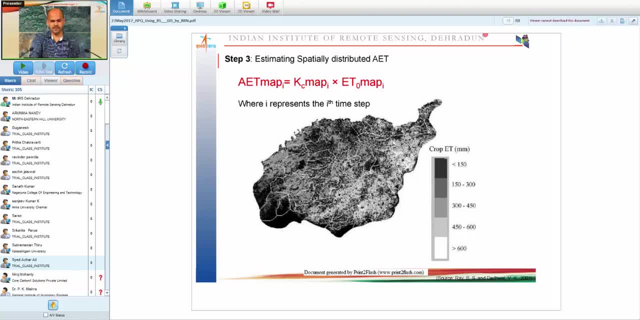 You can get remote sensing data for every fifth or seventh day. If you are in 25 meter resolution, you can get remote sensing data for every 23rd day. So it is still better than the Kc Discretion that is being done. Kc discretion is done if growth stage is divided. is a total growth stage is 120 to 150 days, you can get only 4 Kc values because the growth stage is divided into four stages, whereas now I have for 120 days and if I am choosing five day interval data. 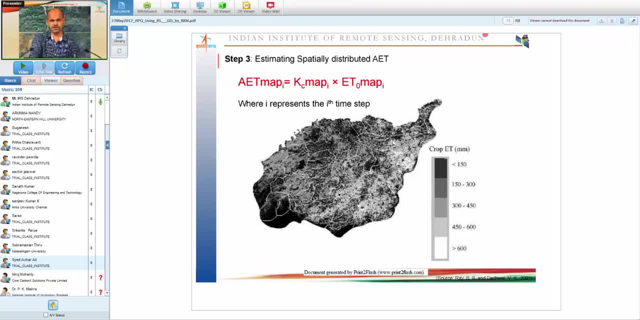 Whereas now I have for 120 days and if I am choosing five day interval data, I will be having 24 NDVI or vegetation index value which I can correlate with the whatever Kc values I have and intermediate values I can interpolate, so I can get for entire growth stage 24 Kc values, which is much better representation in temporal scale and, of course, is a better resolution in special scale. 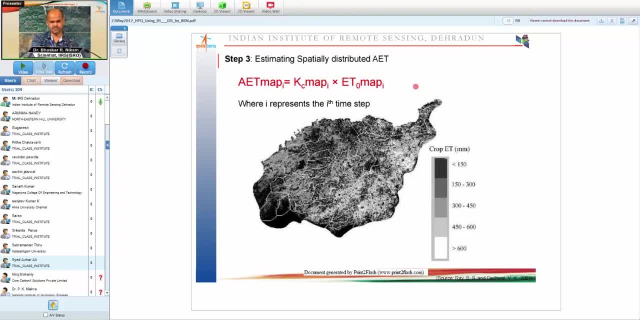 So now, since you, when you have Kc map for a specific time scale, the only thing that you have to do is multiply the reference evapotranspiration map, which is you have generated using interpolation. So when you have Kc map and you will eventually evapotranspiration. the figure here shows the actual evapotranspiration loss from a canal command for that season and, as you can see, wherever I have a healthy vegetation, the evapotranspiration loss is higher. wherever this is a tail reach of a canal command and all those who work in irrigation system know that in a tail reach the crops health will always be a questionable condition. 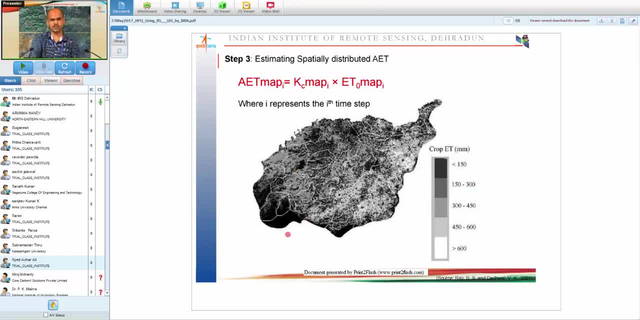 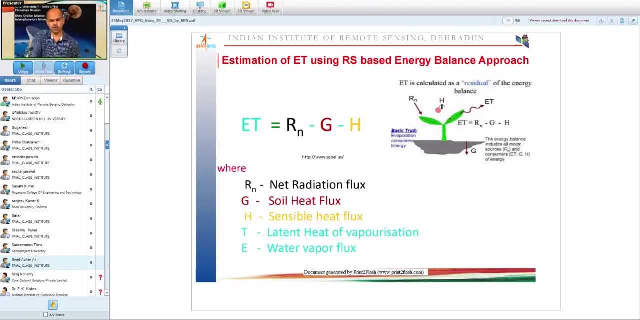 So in a tail reach I have very less evapotranspiration losses, So this kind of product will be useful for many users. Now, this is what we did if we want to fuse the traditional and remote sensing approach. but the problem here is we are still using the point observation to calculate. 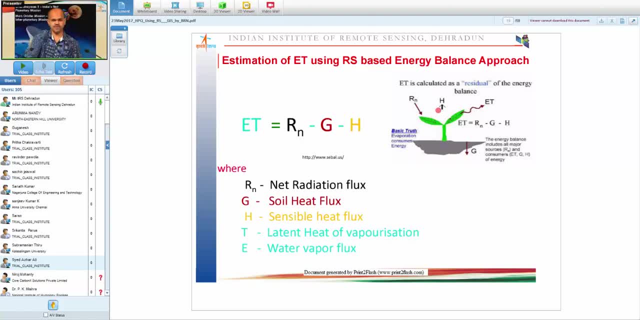 reference, evapotranspiration and, as you know, even the wind speed will not be true. which is you are measuring at a metallurgical observation will not have the same value if I just take offset of 100 meters or 1 kilometer, whereas you know the image, typical 25 meter resolution image will cover area. 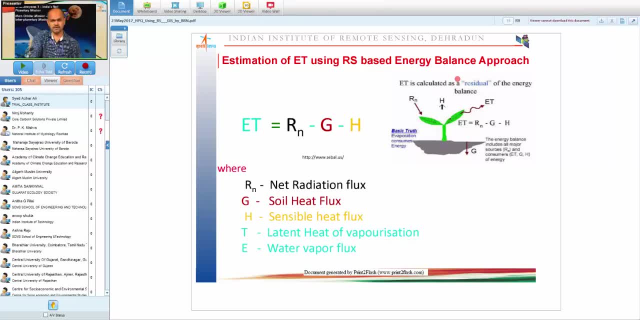 something around 150 kilometers to 200 kilometer. The 25, 56 meter resolution image will cover area something around 750 kilometer, So one or few metallurgical stations may not represent the actual metallurgical situation of the entire area. To overcome that, as I have discussed, there is an alternate. 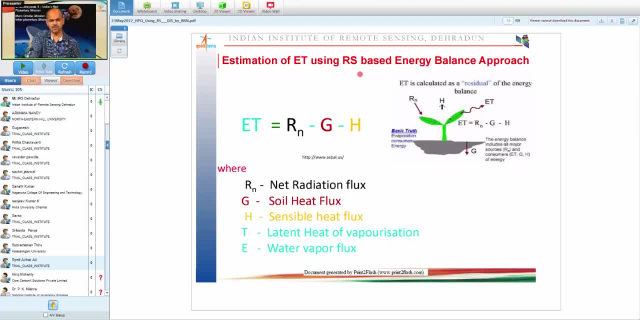 solution which is a metahedral method. The metahedral method is a method of approach which is a much advanced one, where we use remote sensing and we apply the basic energy balance algorithm on remote sensing data. so the basic algorithm says energy used for evapotranspiration. 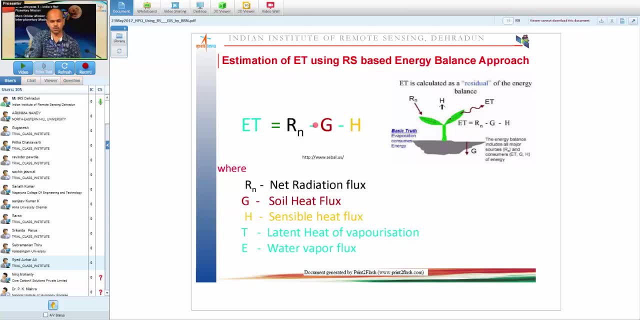 is a residual if I minus the energy used for heating of soil and for heating of air from the total radiation. so this is the total energy that you receive from Sun, minus the energy used to heating up your soil surface, minus the energy used to heating up the used for heating of the air. so the rest energy will be used. 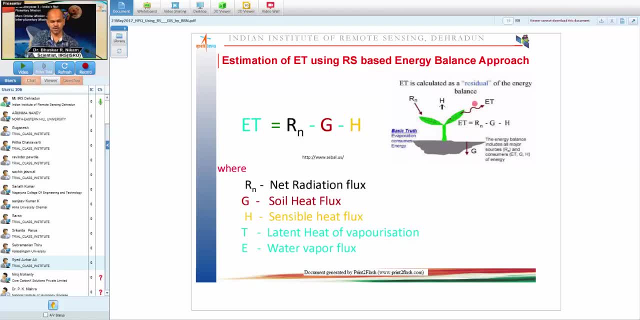 for evapotranspiration only. So this is the energy balance algorithm, which is very, which is represented in this figure. This is the total radiation that you receive. this is the energy used for heating up your air, this is used for heating up your soil, and the rest component is the energy for. 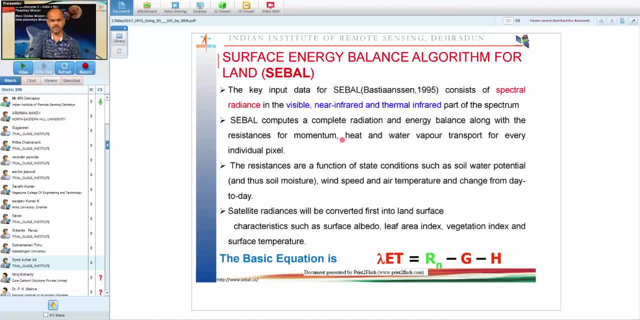 evapotranspiration. now there are many algorithms which use remote sensing data and they perform energy balance estimation. out of them, the most popular one is a surface energy balance algorithm for land, seabull. the advanced version of the seabull is called metric, which is operationally used by USGS for 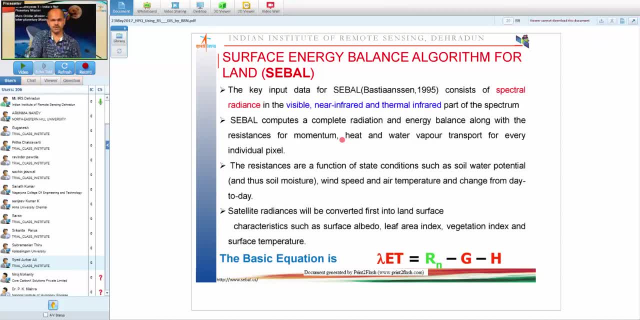 daily or weekly evapotranspiration assessment or entire Northern American continent. the global data of evapotranspiration estimation using seabull or energy balance is also available from modest product. now, the seabull algorithm which we are going to talk only requires the spectral reflectance invisible near infrared and thermal region. it solves all the energy. 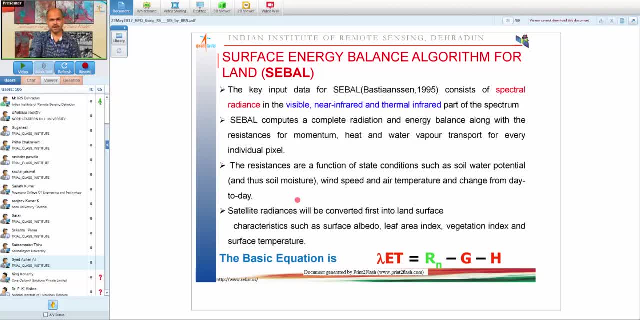 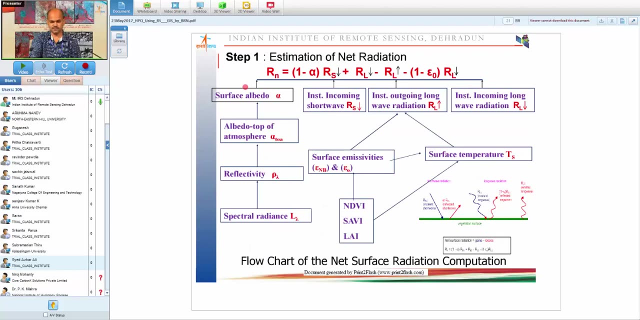 balance subcomponents using remote sensing, 165 00RF for thermal regions data and partially the metallurgical observation. So the basic equation of our discussion is: latent heat of the latent heat, flux of evapotranspiration will be equal to net radiation minus ground heat flux, minus atmospheric sensible heat flux. Now step one would be calculation of 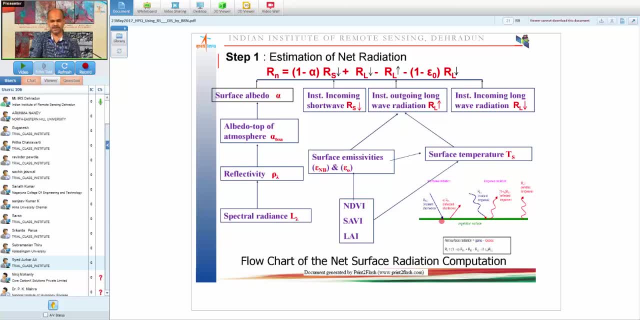 net radiation. As the figure here indicates, net radiation is a vector sum of five components. The first component is incoming shortwave radiation. Because I said it is a vector component, I am going to denote incoming as a positive, so the outgoing will become negative. So once I receive, 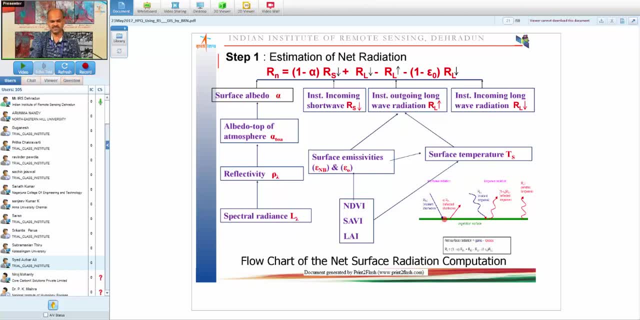 incoming shortwave radiation. two things will happen if the radiation strikes the surface: either it will be absorbed or it will be reflected. Now, if it is absorbed, there are few things happen. it will be transmitted or it will be emitted. but for on a surface, the radiation will be either 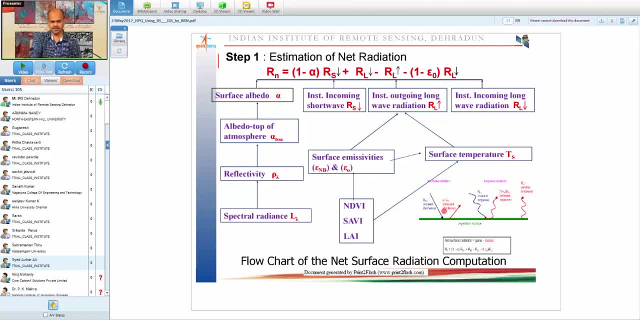 absorbed or it will be reflected. So the first component is incoming shortwave radiation. So the reflected shortwave radiation will be outgoing. So I am representing that as a minus negative. Now I also receive incoming longwave radiation which I am indicating as a positive. 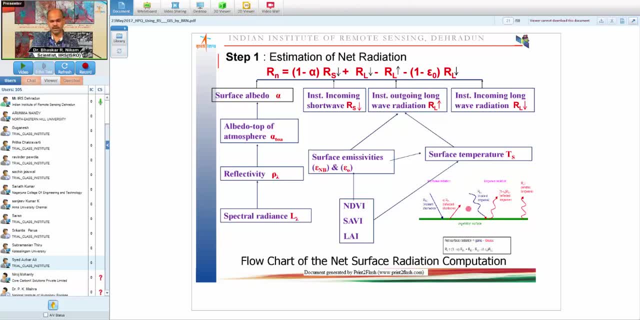 Some part of that will be reflected. longwave radiation and, as you all know, everybody above zero degree kelvin will emit energy in form of electromagnetic radiation and since earth is also having a shortwave radiation, it will be reflected as a negative. So I am representing that as a negative. 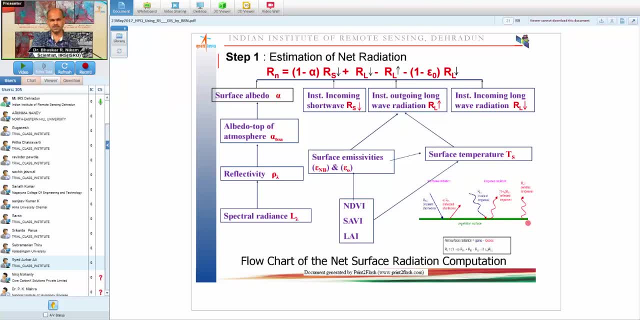 So I am representing that as a negative. So I am representing that as a negative. So I am representing having surface temperature above zero degree kelvin. earth will emit energy in the form of electromagnetic radiation, and the central frequency in which body emits energy is inversely proportional. 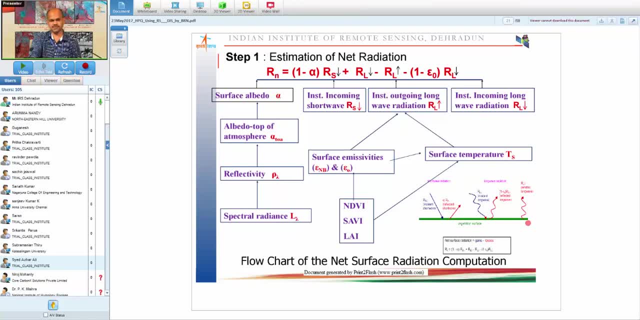 to fourth, power of surface temperature of that body. Since sun's surface temperature is somewhere around 6000 degree kelvin, it emits maximum energy in a shorter wavelength, having central frequency of 0.55 micron, whereas earth's surface temperature is only around 300 degree kelvin. So earth emits 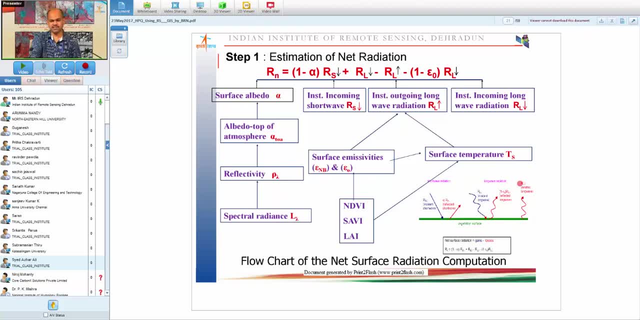 maximum energy in longer wavelength. So this is a longer wavelength which is going out of the surface, going away from surface due to emission. So if I summarize this net energy balance equation, net energy equation it would be net shortwave radiation incoming longwave radiation. 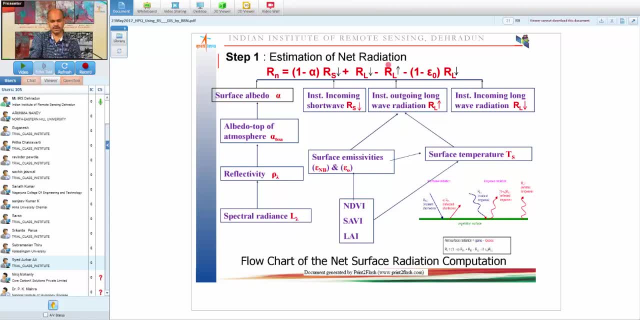 outgoing reflected longwave radiation and this is outgoing- sorry, this is. yes, this is outgoing emitted longwave radiation and this is outgoing reflected longwave radiation. Now, in longwave region like here, this alpha represents albedo. Albedo is a ratio of reflected shortwave radiation to the 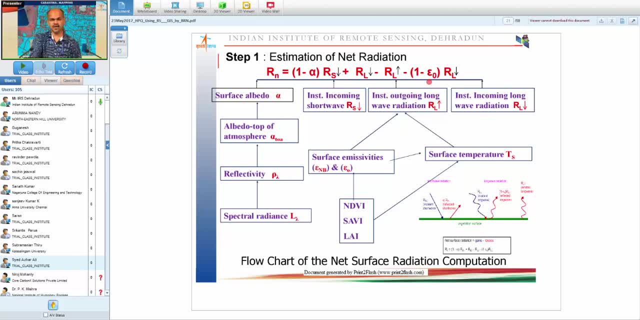 incident shortwave radiation. We don't have same reflectivity term in longwave. So what we have done for instantaneous image acquisition, we are calculating reflectivity by one minus one emissivity. Now this is a reflectivity multiplied by inflected longwave radiation. Now this is a flow. 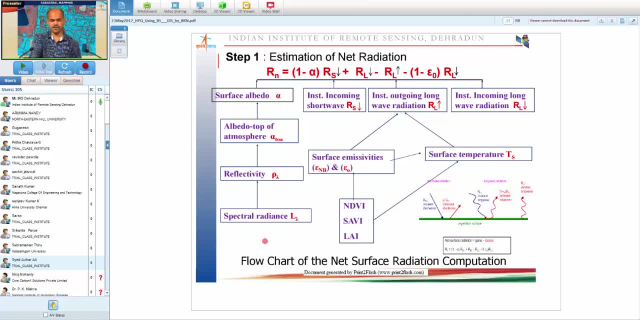 chart using remote sensing data. This is a remote sensing data. This is where I'll have digital numbers. I can convert digital numbers into radiance, radiance into reflectivity and from reflectivity I can calculate albedo at the top of atmosphere If I know the atmospheric transmissivity. 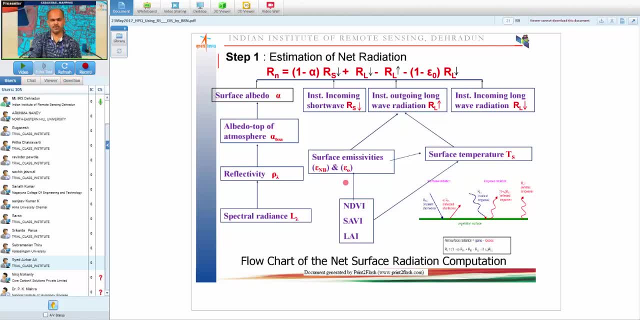 values. I can convert this albedo top of atmosphere into albedo of surface. Now, from those remote sensing data I can also derive vegetation indices which I can correlate to calculate emissivity of the surface. There are various algorithms using which you can calculate emissivity of the surface. You can using thermal data. you can also calculate the surface temperature. 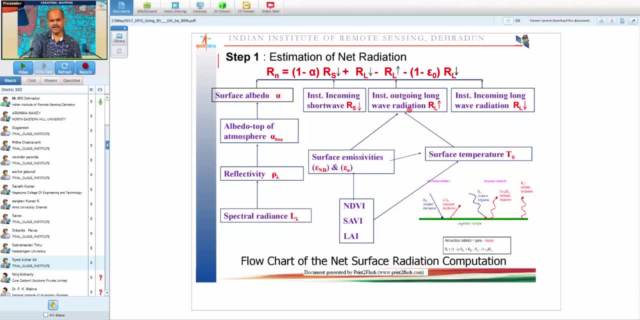 Now if I have a emissivity of a surface and surface temperature, I can calculate emitted longwave radiation. The incoming shortwave radiation depends on day of year, time of day. So it depends on inverse relative distance between sun and earth which day of year 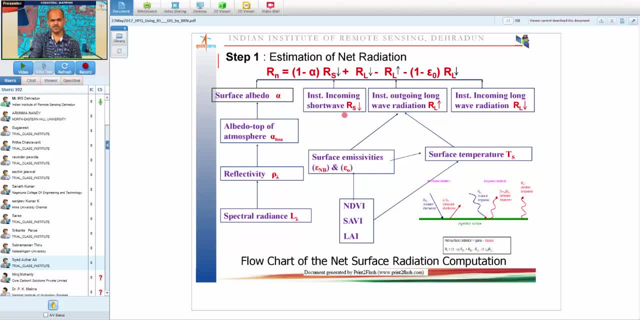 tells me and it depends on the inclination angle which the time of acquisition of image tells me. So the shortwave radiation will be constant for that specific time. So if I have albedo and incoming shortwave radiation, I can shortwave radiation part. Longwave radiation will come towards my 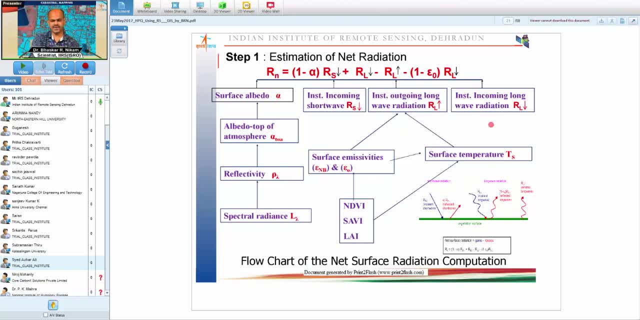 surface because of air temperature. So this is where satellite lags in giving air temperature. But we'll try to resolve it using some anchor pixel algorithm we'll discuss in coming slides. So just assume that we have a air temperature So we can calculate air emissivity. I can calculate. 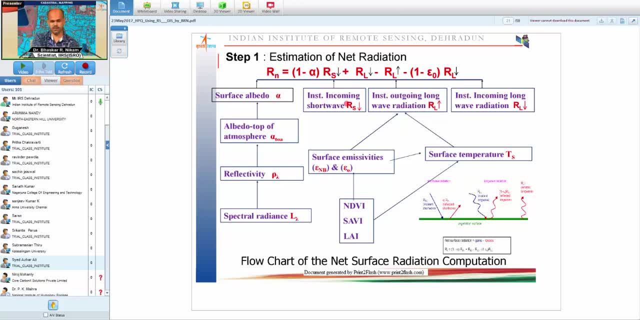 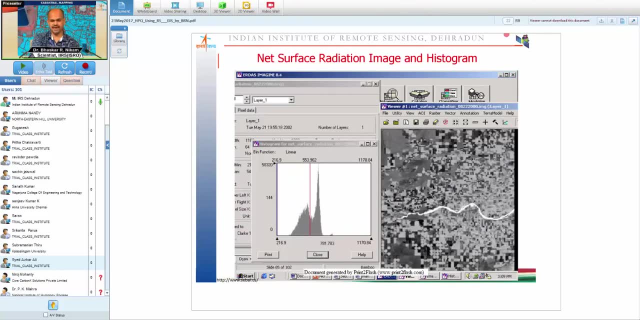 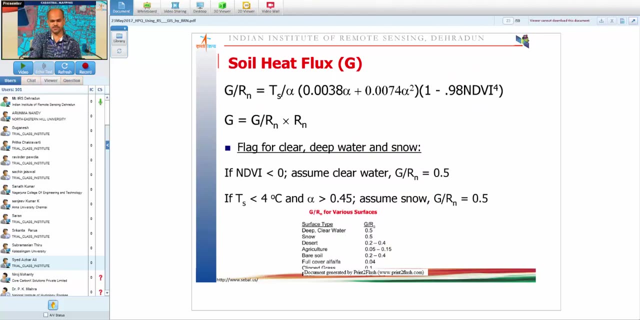 incoming short longwave radiation. If I have a surface temperature I can calculate the emitted longwave radiation And if I put those values here I can get the net radiation that my surface has. So this is a pictorial view of net radiation estimation. Now, out of that net radiation some 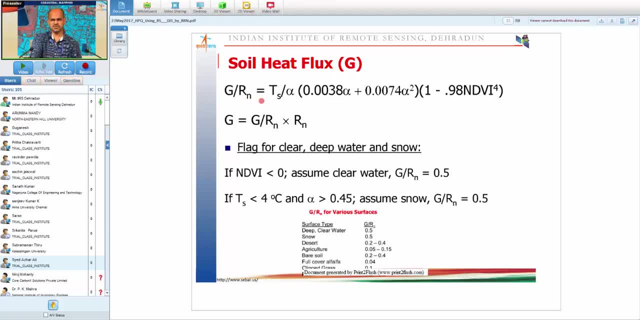 part of that net radiation will be used to heat up soil or heat up surface. There are very simple or simplistic equations. if you have surface temperature, albedo, vegetation indices, you can calculate the energy used to heat up surface as a ratio of soil heat flux divided by net energy. Even in traditional 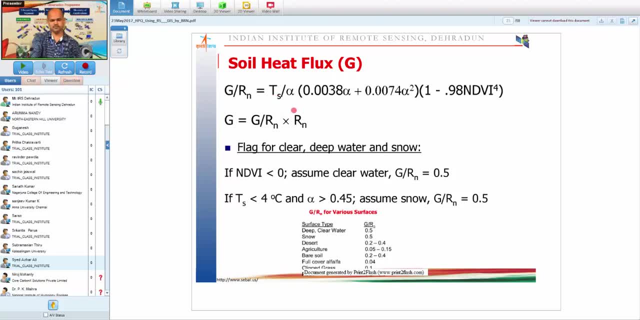 metallurgical ET estimation approach. also, we calculate this ground heat flux using the same approach, G by Rn ratio. where you require in this specific algorithm, you require surface temperature, albedo and vegetation index. Now we also have to account for specific surfaces, like which generally will have higher albedo. 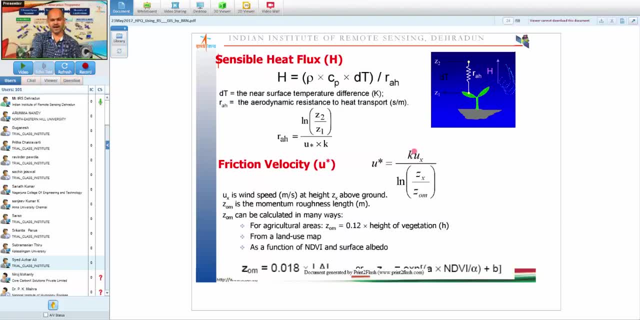 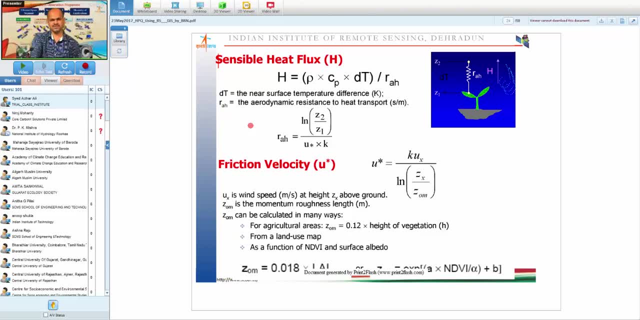 we can calculate the energy used to heat up the soil. So we can calculate the energy used to heat up the soil. So guardian class class with typical G by Rn ratio. Now, the only unknown in our basic equation is Sc Consulting. Sensible heat flux of atmosphere can get calculated if you do. 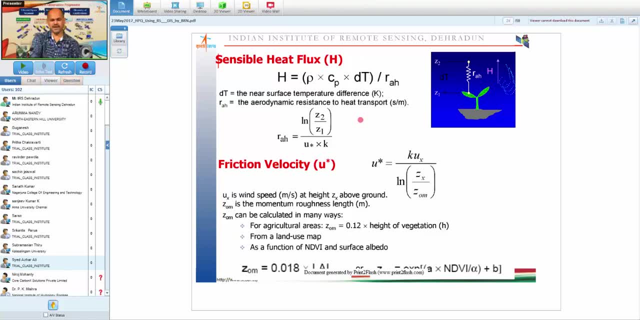 données de peso con el temperatura urbano. This Dt is the temperature difference between the surface and the air near theuber fulfilme and RHcoal HahE surface and Italy and areause aie in error dynamic nastos to heat tr tr dt. Whether. 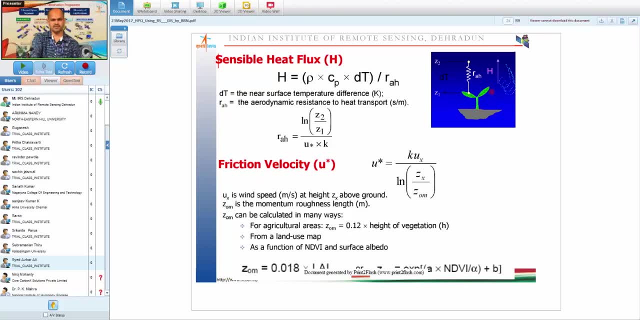 manifests in Eck. We do not know the aerodynamic resistance of the surface. the roughness can be ignored. But if it is a vegetated surface the roughness values will vary tremendously. So we cannot ignore this Now. dt is the temperature difference between the surface from where evaporation is happening. 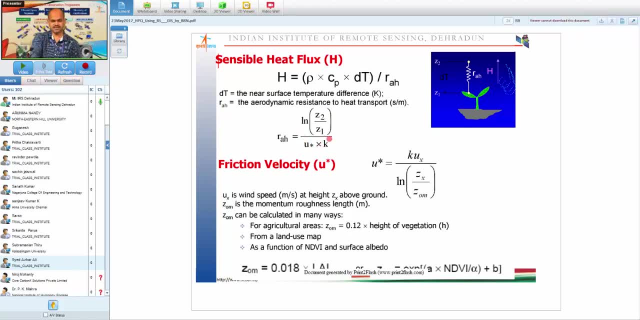 and the surface near the air, near to that surface. So this aerodynamic resistance can be calculated if I know the frictional wind speed, and this k is a Von Korman constant which has a value of 0.41.. But for that I need this z1 and z2 heights, where the RAH will play a role. 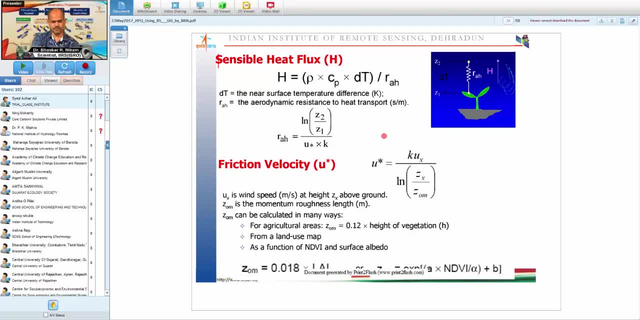 This we can calculate if we know the height of vegetation. But what we measure in meteorological observation is the wind speed at specific height. It could be wind speed at 2 meter, wind speed measured at 3 meter, wind speed measured at 5 meter. 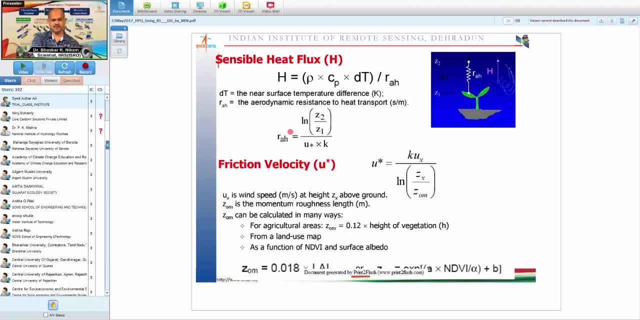 We don't measure the frictional wind speed From the measured wind speed From a meteorological observatory. we have to calculate frictional wind speed so that I can calculate aerodynamic resistance and then I can, using some more algorithm, I can calculate this near surface temperature difference so that this sensible heat flux of air can. 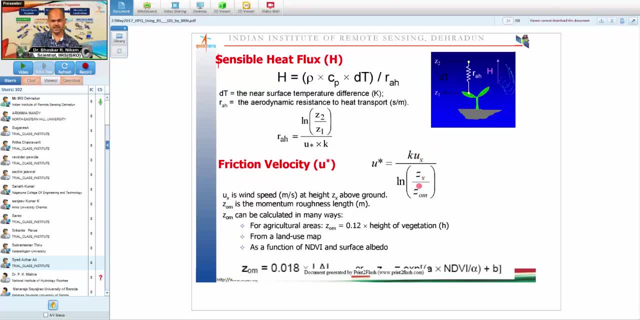 be calculated and our equation can be solved for calculation of evapotranspiration. Now, frictional wind speed can be calculated, if I know the wind speed measured at x height, the momentum roughness length, which is a function of vegetation height, And people have tried to correlate this with LAI or NDVI. but what I am trying to emphasize, 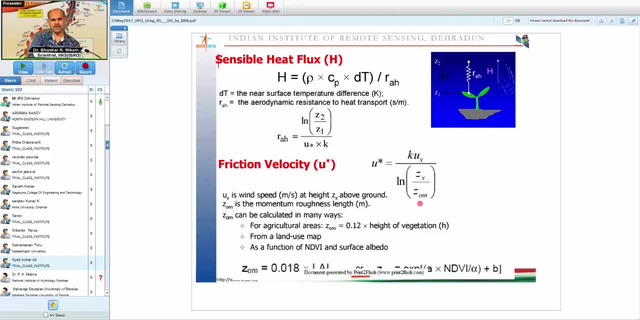 here is ZOM is a function of vegetation height. The vegetation in entire area will not have same height, so I will have different frictional wind speed at different, different locations, which we necessarily said why we should go for traditional approach. Now, to calculate this winds, frictional wind speed, I need wind observations. I will have. 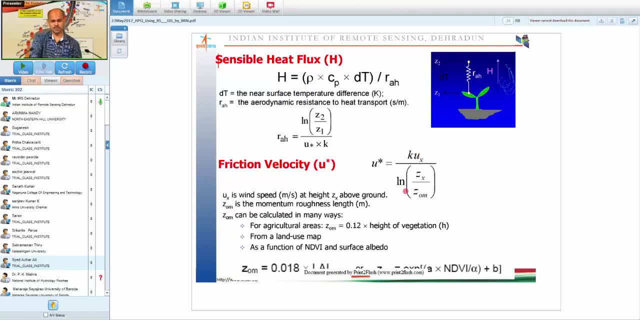 for one point only. But as we all said just a moment ago, that for a point where you have this wind speed observation, ZOM will have some value. but if you move away from that point, ZOM will vary. So the wind speed, or frictional wind speed, which I am calculating from the meteorological 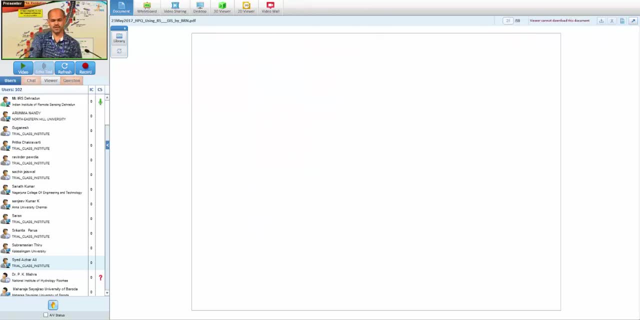 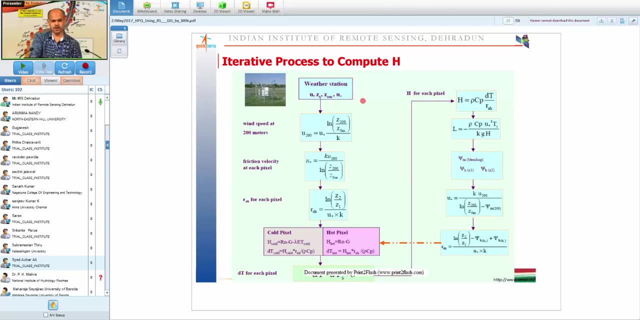 observatory, will not be true for the adjoining pixels or far away pixels, So we will try to solve this in a iterative algorithm which is represented here. So for a meteorological station, this wind speed and all other parameters are observed. So I will convert and since I know the wind speed measured at meteorological observatory, 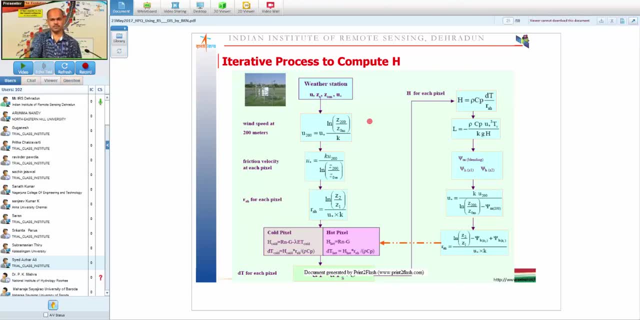 at is a 2 meter height or 3 meter height or 5 meter height, and which will not be constant in other pixels. so I need wind speed option for that pixel to. I will convert wind speed measured at 2 meter height to wind speed measured into 200 meter, for which I will use the frictional. 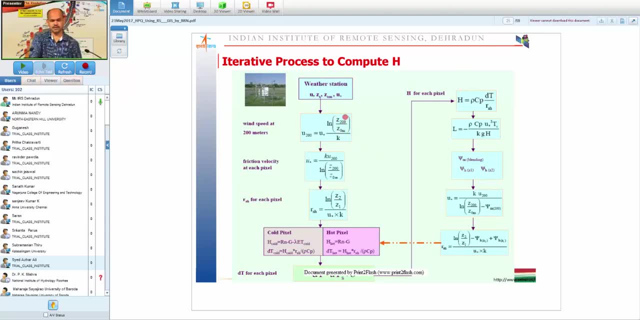 wind speed. ZOM is a momentum roughness length. this is a 200 meter and this is a Von Korman constant. So now for the meteorological observatory. I have converted a wind speed measured at 2 meter to the wind speed at 200 meter and I am assuming right now that wind speed at 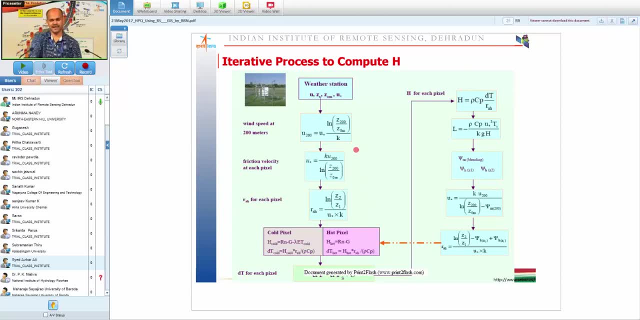 200 meter will remain constant for all my pixels, all my entire area. With that assumption, I will calculate this frictional wind speed for all my pixels because, see So, since this U200, which is a wind speed at 200 meter height, will remain same for all, 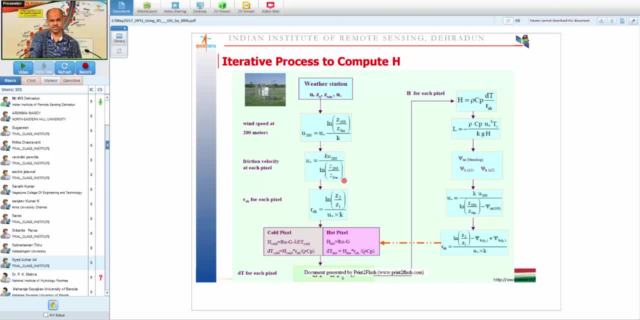 the pixels. but this ZOM is a function of vegetation height which will change for every pixel. So necessarily I will have different frictional wind speed at all the pixels and since U star is different, the RH for all the pixels will be different, which is a aerodynamic resistance. 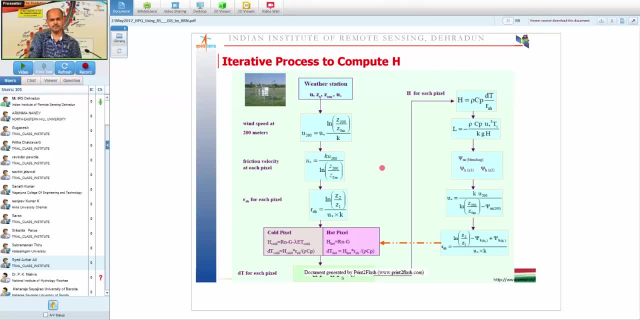 for heat transfer. Since RH is different, my sensible heat flux of atmosphere will be different. At this moment, let's assume for all the pixels we have this RH value, but I am still not having the DT value, the temperature difference between surface and air, to near that surface. and since, 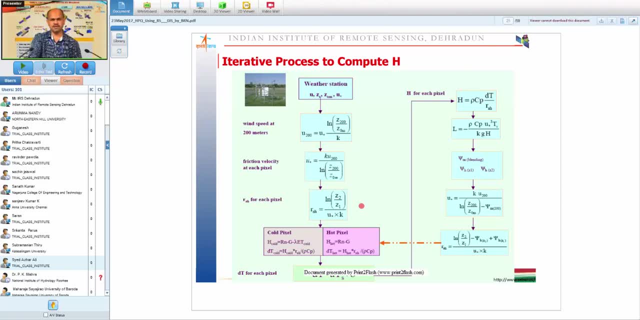 I told you that light will not give me the temperature of air near to that surface. So we in this algorithm, rely on an anchor pixel algorithm where I will search, or a user will search, a cold pixel and a hot pixel in a 50 degree angle. 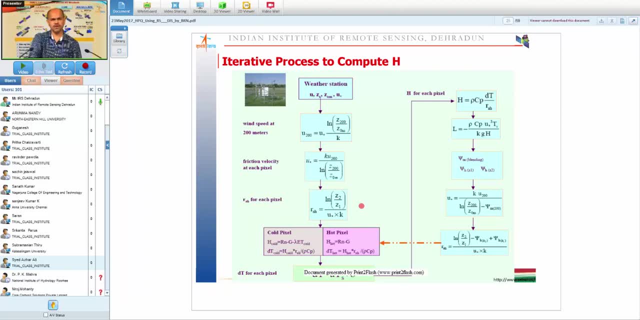 And I will find a pixel in a 50 kilometer radius or 500 meter radius from your metallurgical observatory, depending upon your special resolution of data. Now, when I am saying cold pixel and hot pixel, I am referring to land surface temperature of that pixel and I am not talking about the coolest and hottest pixel I am talking about 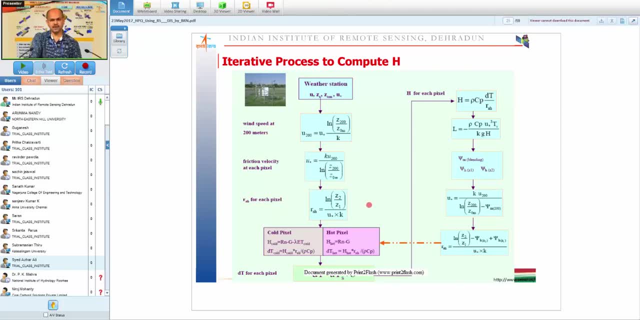 cold pixel and hot pixel. Here we assume that the pixel which I am designating as a cold pixel will have a lesser surface temperature value, Because the pixel has a healthy vegetation and it has ample amount of water, due to which maximum energy available in that area is used for evapotranspiration. 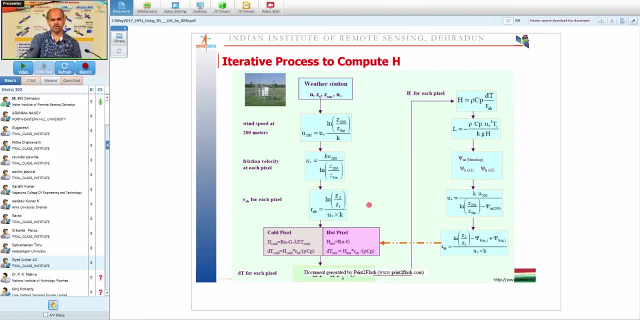 So less energy is used for heating up the soil, whereas on the other hand, in hot pixel I may not have vegetation, so the transpiration part will be missing. I also may not have water in that surface, or will have very less water, so energy used for evapotranspiration will be very less. 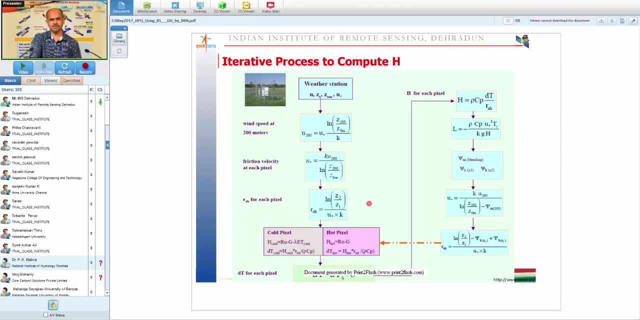 As I discussed in previous section, that around 77% of energy at any given time will be used for evapotranspiration. So you can imagine, if that 77% energy is not used for evapotranspiration, only two things can happen. Some part of that energy will be used to heat up atmosphere and some part of that energy 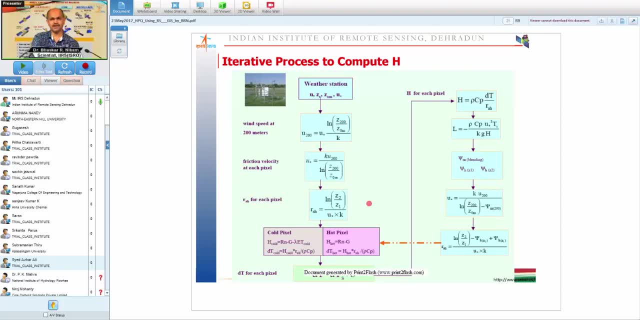 will be used to heat up surface, due to which my surface will have higher land surface temperature. So these two are my hot pixels and cold pixels. So those pixels, we can understand that if it is a hot pixel, evapotranspiration will be zero and if I put this value in my base equation, the equation will become zero is: 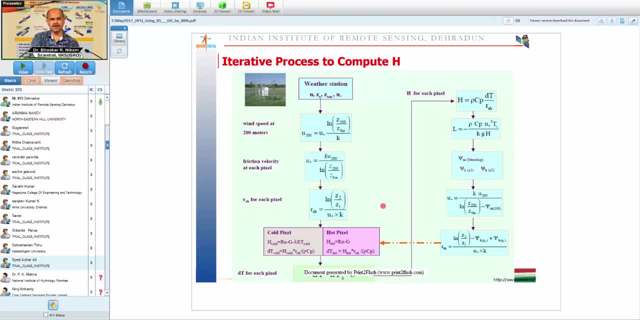 equal to Rn-G-H. Now I have one unknown in H which is DT, but I have on the left hand side I have value zero again for the cold pixel. I can calculate evapotranspiration using metallurgical observations and I can convert them into actual evapotranspiration, taking into account the Kc part. 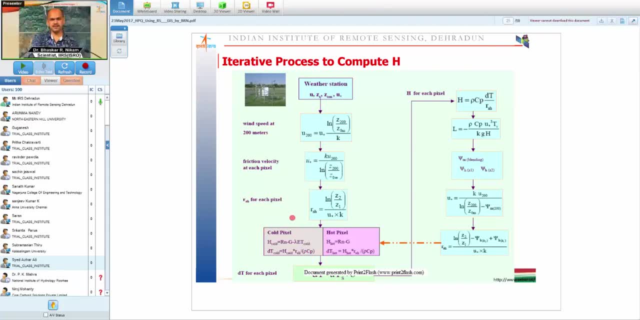 or I can assume that for this pixel the Kc is 1.. So this gives me the actual evapotranspiration from that pixel and that numerical value I can put in my algorithm. So this gives me some numerical value. is equal to Rn minus G minus H Rn. you already have calculated for that pixel G you. 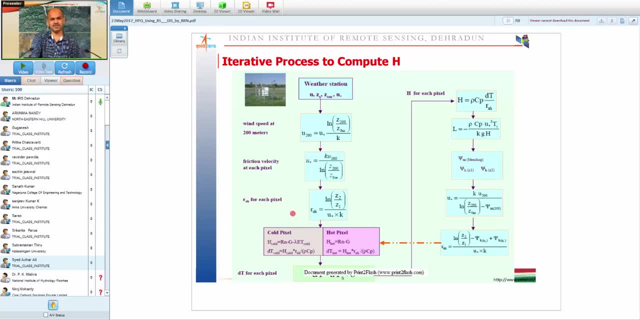 already have calculated for that pixel. So only unknown is H, and within H there is only unknown, which is Dt. So now I have one unknown Dt for two points, hot pixel and cold pixel. So you can solve these one unknown using two known points. So I will get- excuse me, I will get value of Dt for. 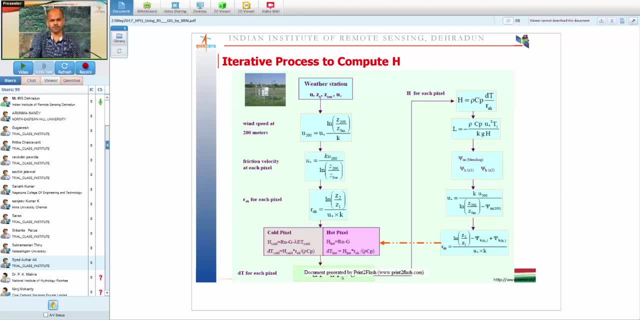 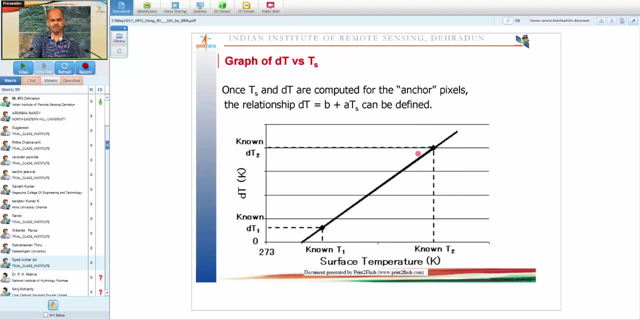 cold pixel as well, as I will get value of Dt for hot pixel. Now I will try to correlate Dt for cold pixel. So I will try to correlate Dt for hot pixel. So I will try to correlate. this is assumption of cold pixel and hot pixel. I will try to plot the surface temperature of 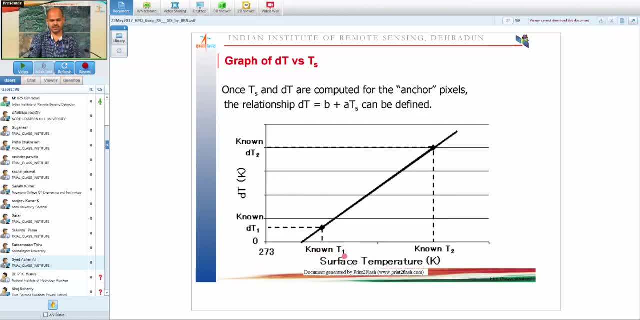 those pixels against the Dt values. As you can see, the cold pixel will have less Dt values and hot pixel will have higher Dt values, and we have selected the cold pixels and hot pixel to represent the pixel having highest evapotranspiration rate and the pixel having lowest evapotranspiration. 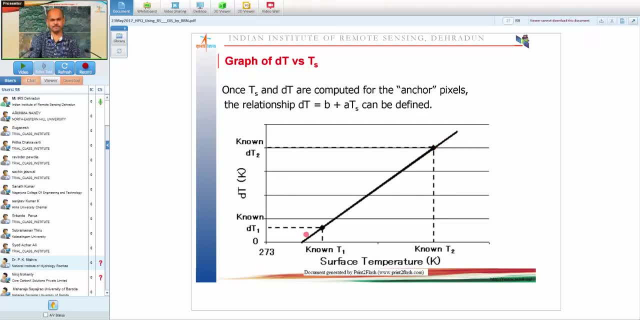 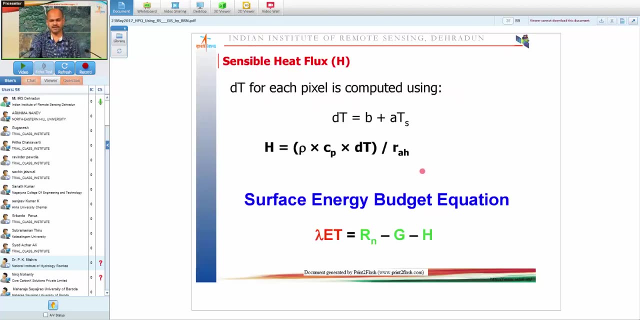 rate. So all other pixels will lie within this line. So I can convert, I can join these two points by a straight line. I can use this equation to convert my surface temperature observations into Dt map. So once I have that, once I have this equation, 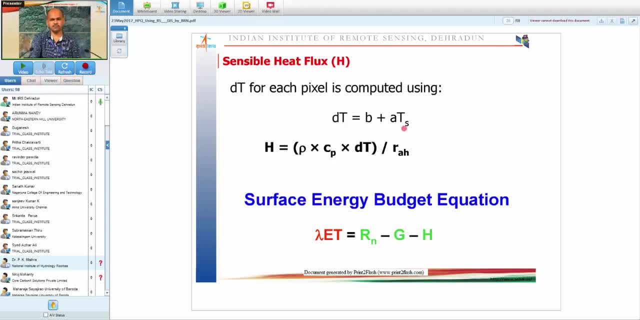 I just have to put in this equation into any software where this equation, this intersect slope and the surface temperature value of every pixel will be given, and that software will give me the Dt value. If I do that, Rh is already known, Dt. I have calculated Rho and Cp is known, So H will be. 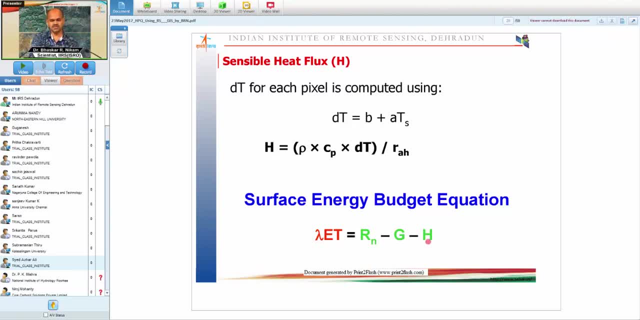 calculated. If that is the case, all the three unknowns in this equation, for every pixels, will be solved, So you will have value of net radiation. You will have value of ground heat flux. You will have value of atmospheric sensible heat flux, So you can calculate energy utilized for evapotranspiration. 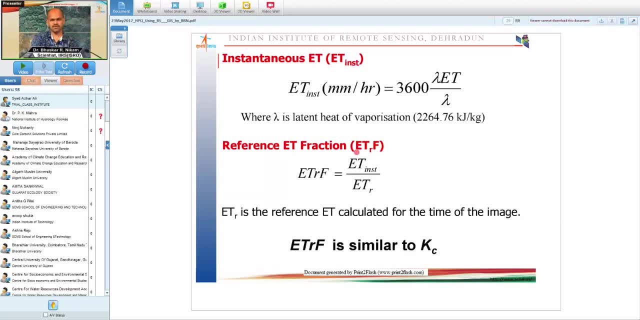 But we are still stuck up with a problem that we, a general user, don't require: the energy calculation. The general user requires the evapotranspiration in terms of volume or weight. So what we will do, we will divide this heat flux of evapotranspiration by latent heat of vaporization. 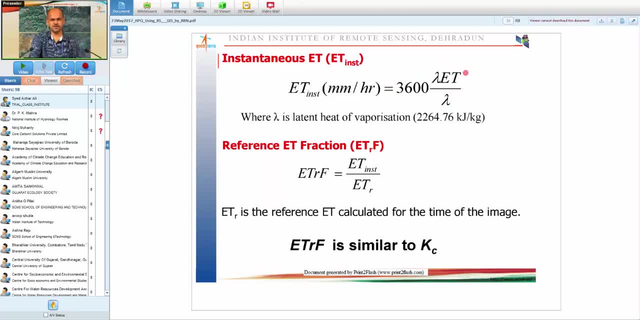 and we are multiplying it with number of seconds in R to convert this observation, because remote sensing is an instantaneous observation. it only represents a surface or energy balance for that specific second for which the observations are taken, Whereas the metallurgical is ET that we have calculated is calculated for 1R. So we will convert this flux used for 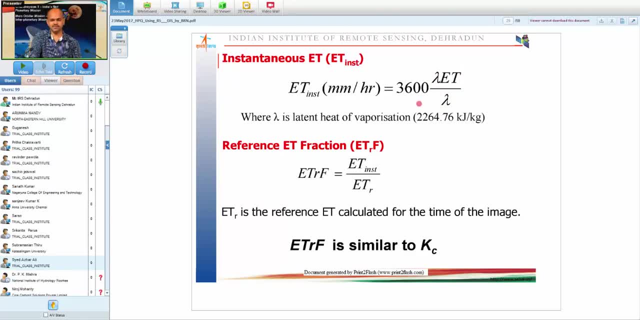 evapotranspiration. We will divide it by latent heat of evaporation. We will multiply it number of seconds in R, So that will give me the instantaneous evapotranspiration rate in mm per hour. Now, this is also instantaneous evapotranspiration rate. Please understand this net energy balance. 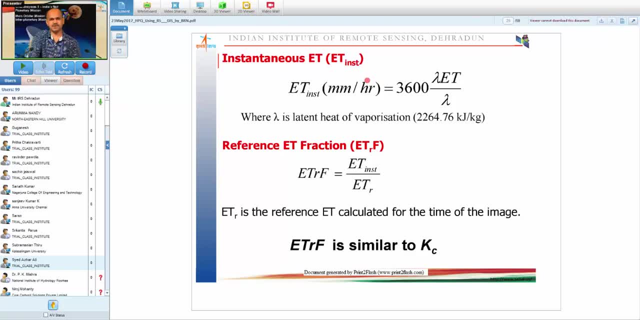 this Rn that we have calculated is true for that specific time only If? because the net energy, the shortwave radiation that we receive depends on inverse relative distance between sun and earth and also it depends upon sun's inclination angle, which changes with day of time, day of 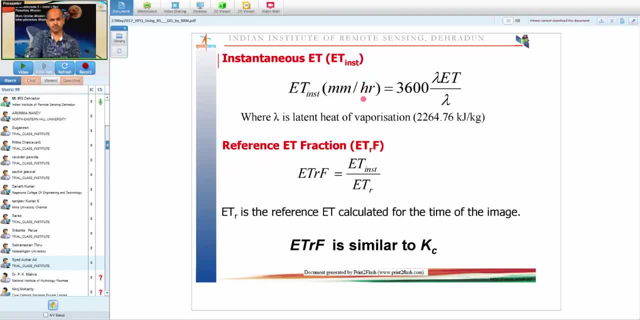 sorry time of day. sorry So because with time of day the inclination of sun will change, So my Rn will change, So the entire energy balance will change, and so my Et will also change. So I can use this instantaneous Et for representing instantaneous evapotranspiration from a surface. 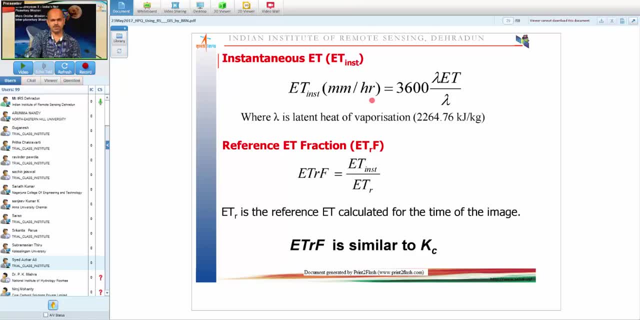 for that instance only, Whereas this- any Et estimation- requires daily or weekly or fortnightly, monthly or maybe seasonal evapotranspiration estimation. So what we do here is we convert this instantaneous Et into evapotranspirative fraction by dividing reference evapotranspiration. 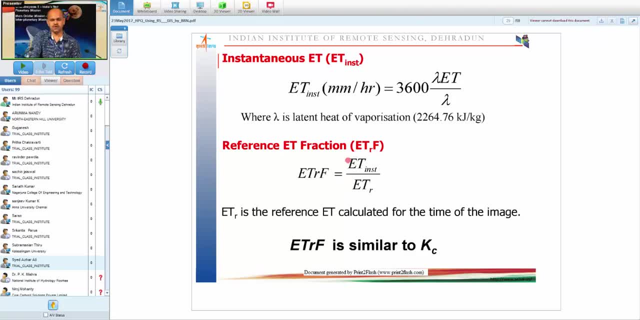 of that time period. So if you want to convert this instantaneous Et into evapotranspirative fraction, So you need a daily Et multiplication factor. So I divide this instantaneous Et of every pixel by this reference evapotranspiration which you have calculated using metallurgical. 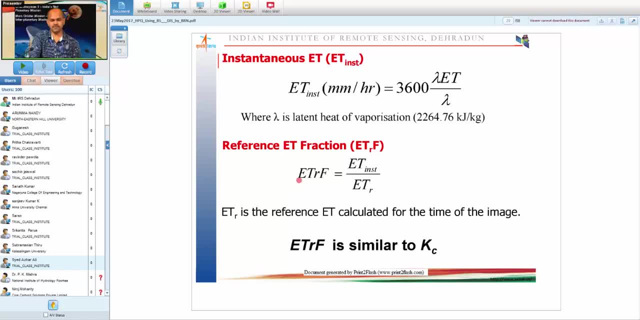 observation And this is what we call EtRF, reference reference evapotranspiration fraction, And the formulation of reference evapotranspiration fraction is similar to crop coefficient, See this reference evapotranspiration fraction tells you that what is the difference in actual Et compared to reference Et? And this difference will be only because of physiological 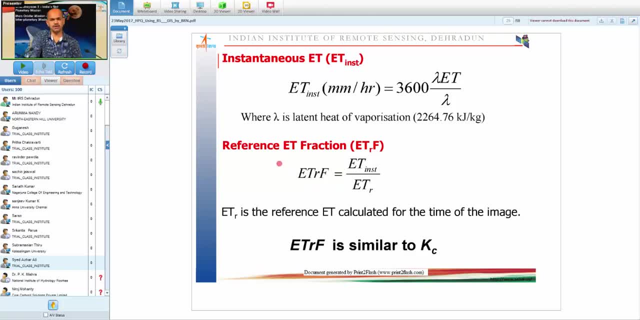 parameters of your surface and biophysical parameters of your vegetation. So remote sensing also gives you KC advantage. here is because I can get remote sensing data for every three day, four day or maybe Now We have advanced constellation of satellite We can get remote sensing data even for daily. 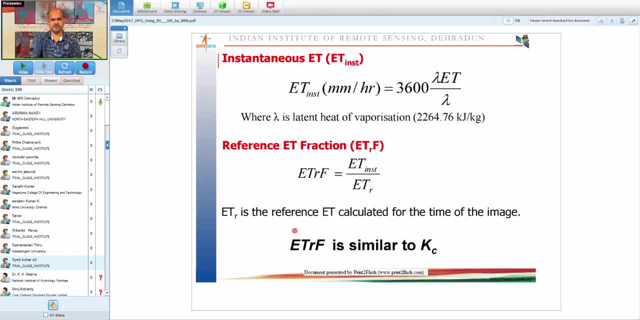 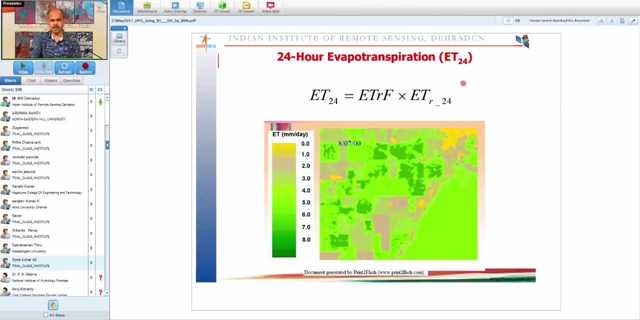 at five or sub, maybe three or four meter resolution. So now I can generate these KC values for a specific crop at three, five or ten days interval. Earlier we used to have these values at a very discrete intervals. Now you can convert this using this EtRF. you can convert your. 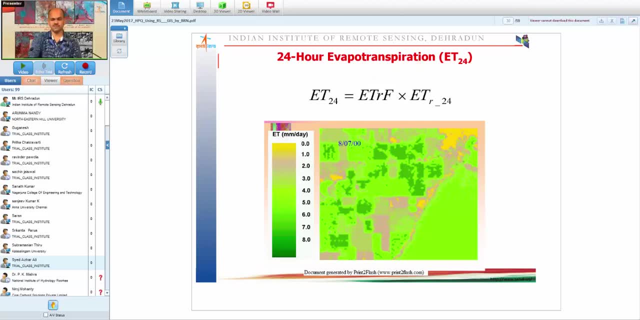 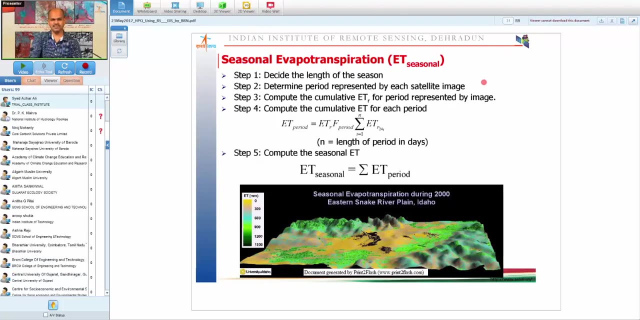 reference evapotranspiration into daily evapotranspiration or seasonal evapotranspiration. There are few steps That you have to understand in seasonal evapotranspiration. First thing, you have to decide the season, the time period of the season, and choose the images which represent that season most appropriate. 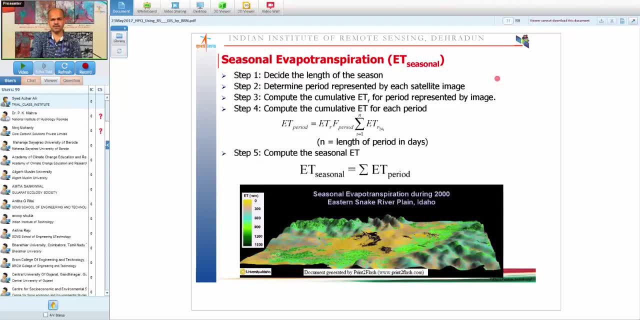 would be the season The images should represent the divisions, like if I am doing it for January, preferably the image should be from the middle week of January. then calculate the EtRF for that period. ETRF for that period multiplied by the ETR of that period, you will get ET of that period. 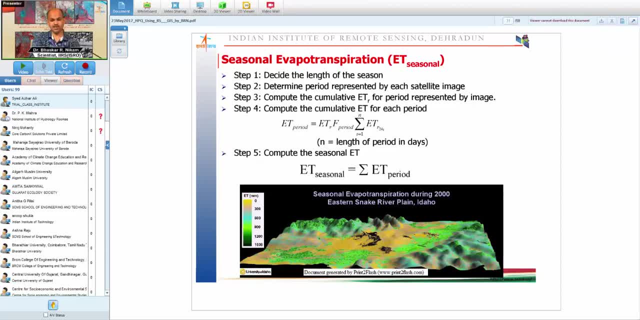 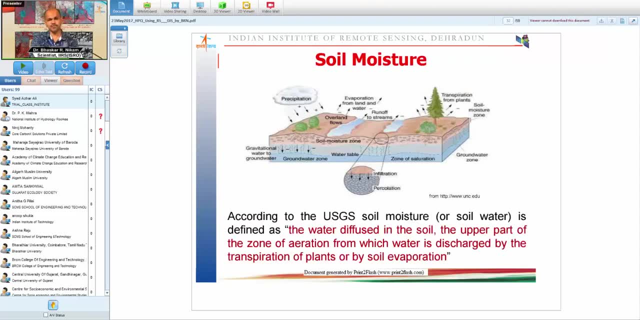 So this graph here shows a three dimensional plot of actual evapotranspiration loss from a season from the experimental field in US. Now we are coming to the last section of our presentation: soil moisture. Now I will rush through this because I think time is limited. 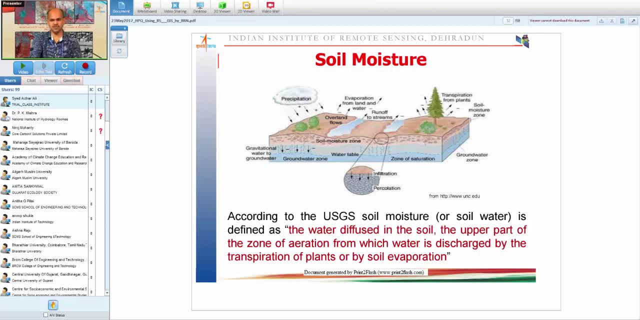 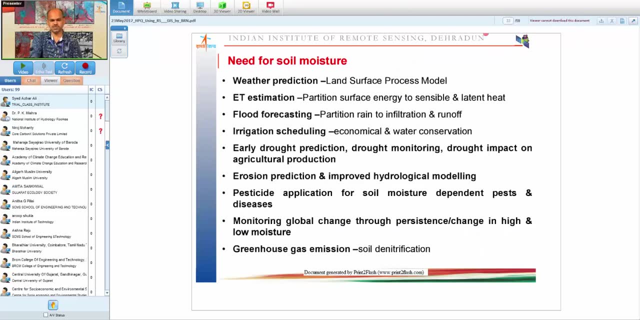 As we all know, soil moisture is a water stored in the upper zone of aeration which will be used by vegetation for evaporation, and also it will be lost by sorry, which will be used by vegetation for transpiration and lost by evaporation process. Now soil moisture is termed as essential climatic variable in terrestrial section because soil 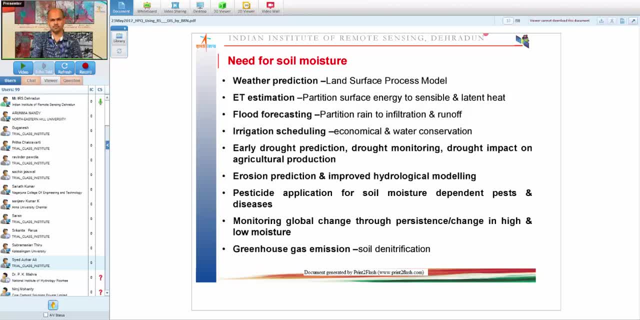 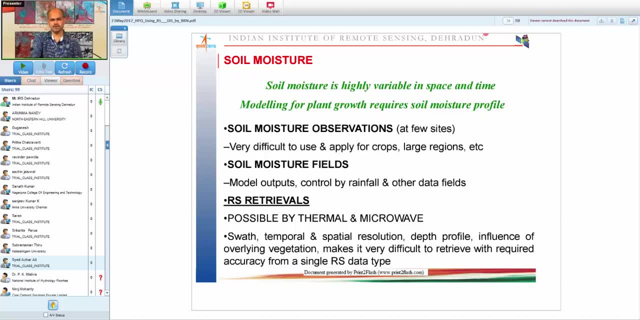 moisture governs your energy exchange, as well as what you can say mass balance between atmosphere and land surface. So observing soil becomes very important. But the problem with traditional observations are they are point based. They are either very time consuming and laborious or they are very costly. whereas remote sensing, 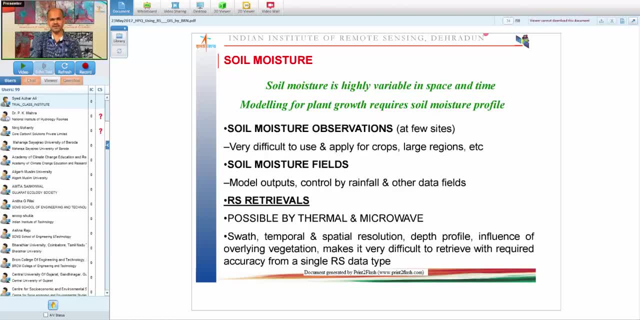 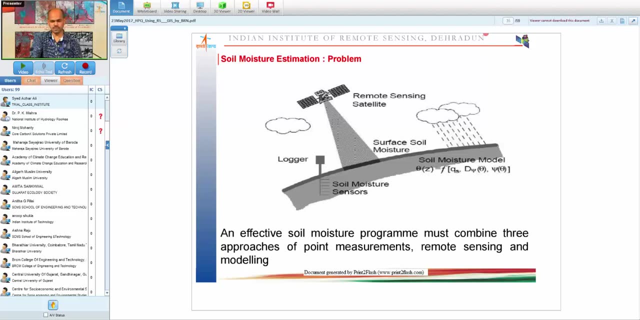 has advantage of synoptic and repetitive coverage. So people started searching. can remote sensing be used for mapping or monitoring soil moisture? So all forms of remote sensing, including active, passive or optical, thermal and microwave, are used for soil moisture mapping. The typical robust algorithm of soil moisture estimation should include all the three components. 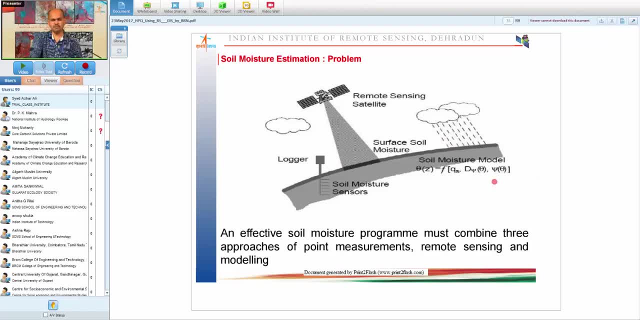 The remote sensing component, the field based observation and the model. Why it should be, As Dr Praveen told you, that no matter how big your constellation is, remote sensing satellite gives you a snapshot of a specific time period, whereas let's say once in a, two days, once. 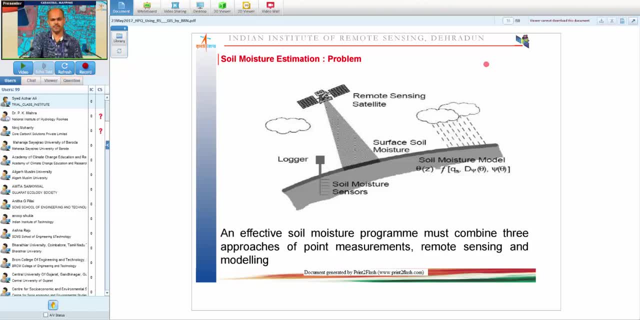 in a week or once in a seven, maybe ten days. So it is very important. But, as you know, soil moisture is a specially varying phenomena with time and space. So the dates between which I don't have these satellite observation, it is very difficult to interpolate the soil moisture of that specific location. 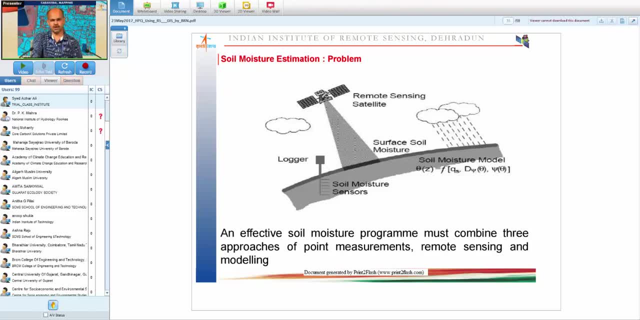 Again, satellite may not cover all the locations of earth in one day or when the satellite is passing some local event. Dr Praveen Choudhary, MD. Okay, Okay, So the data which is recorded by the traditional observations may not be recorded by the satellite? 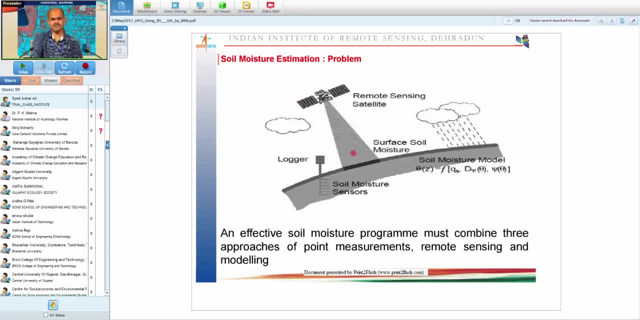 and whatever you are deriving from satellite needs a validation for which you can use the ground based segment. So all the remote sensing based hydrological parameter retrieval algorithms always suggest that those algorithms should have three components of satellite segment, then the modeling approach and the field based observations. 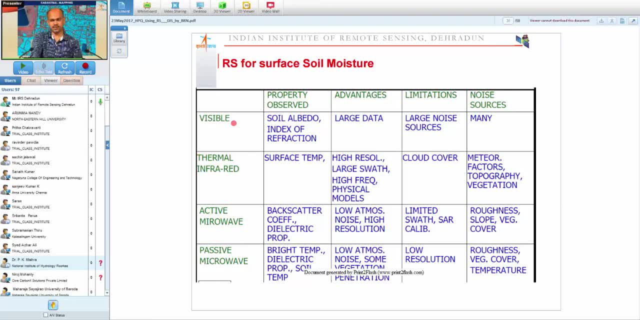 Dr Praveen Choudhary MD. Okay, Now, here you can see we have applied. or the over time visible thermal active and passive microwave is being used in soil moisture monitoring In optical. the problem is we seldom get bare soil and if we are getting bare soil, we are. 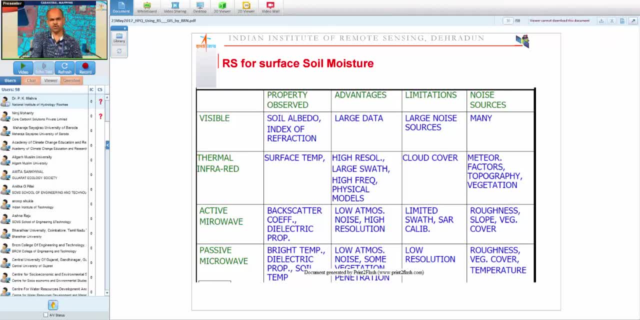 not interested in the soil moisture of that area. We get bare soil in the desert but we never bother about soil moisture of a desert. and if we have soil moisture, with time there will be vegetative coverage on the soil. So that is the problem with optical data. 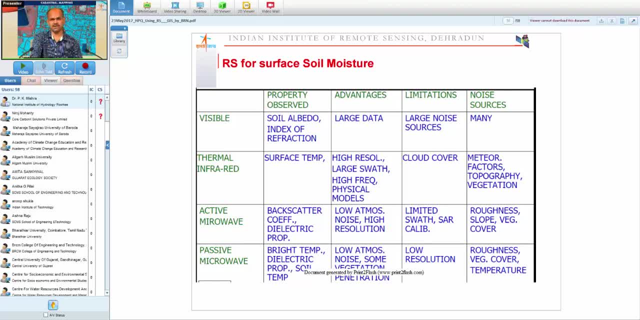 The advantage of optical data is large amount of data is available for a very long time period. With thermal the advantage is thermal represent a combined signature of vegetation surface as well as the soil surface. So if my soil moisture is high, the brightness, temperature or the energy emitted by surface 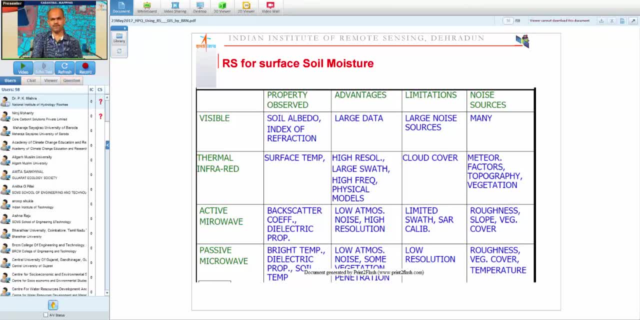 will be less. But the problem is it is very difficult to segregate the soil moisture. So the problem is, if the soil moisture is high, the energy emitted by surface will be less. So rather than segregating this signal from vegetative surface and signal from soil surface, 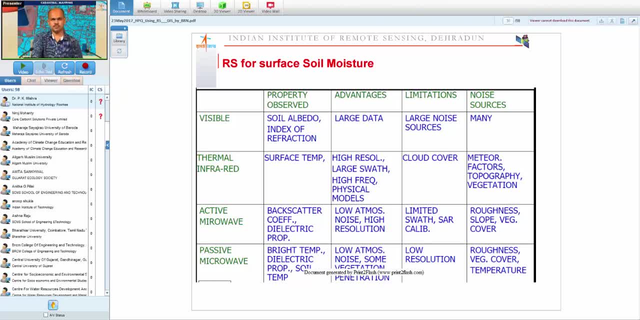 though there are some algorithms to segregate them, But accuracy will be much poorer in case of dense vegetation. Now, active microwave has a tremendous potential in soil moisture from a point of active microwave and penetrate through vegetation. Then the problem with optical and thermal is: if there is a cloud, you will not get data. where, as in active microwaves, you can get data, even there is a cloudy condition. So let us talk about只有 visible and visible, Bella. So as the sometimes I feel glassy light, here I get it, you see, in black and quickly I get. 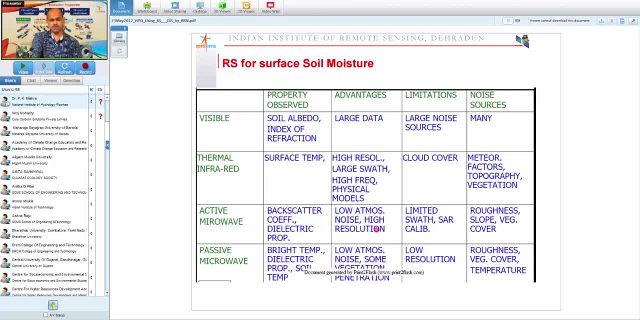 hij Weber, even if I was a very, a very regular conocly one, you were having other visitors. I Заure. so if I draw services I see blue colors but you have higher activity compare to quando I see then this is very sensitive to soil moisture. so even a minor variation in 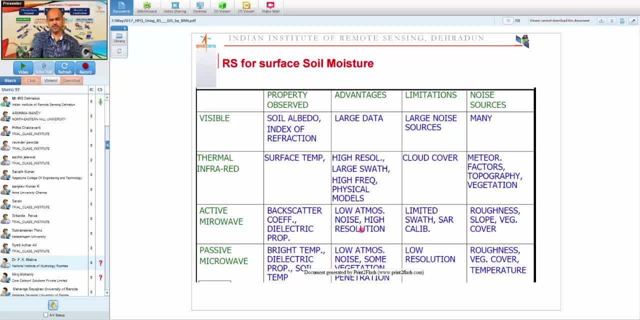 soil moisture can be quantified using of active microwave. the disadvantage is active handling active microwave data is bit difficult compared to all other format and since active microwave is very sensitive to surface roughness, so and surface orientation also, so correcting the data for these parameter becomes much more difficult compared to other, whereas the passive microwave 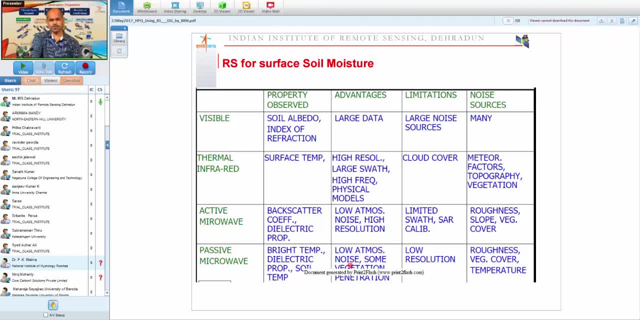 carries the advantage of microwave system, with only disadvantage that it will represent a coarser resolution of 25 millimeter or 36 kilometer area, whereas the limitation of active microwave will not be there in passive microwave, because the signal that we are receiving is a combined signal of a 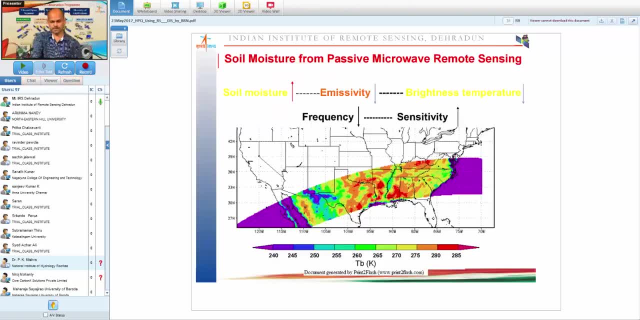 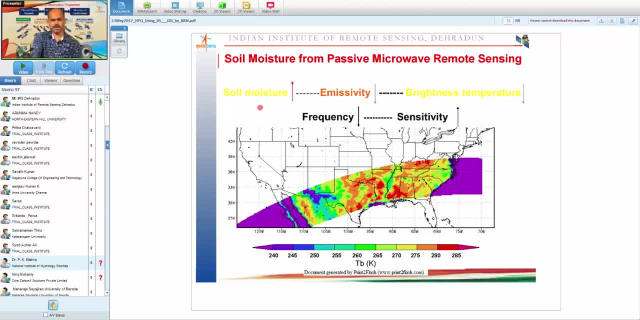 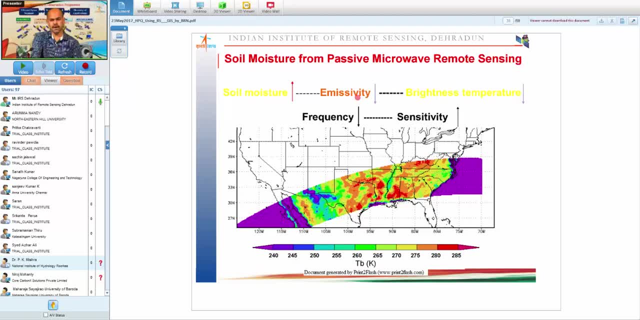 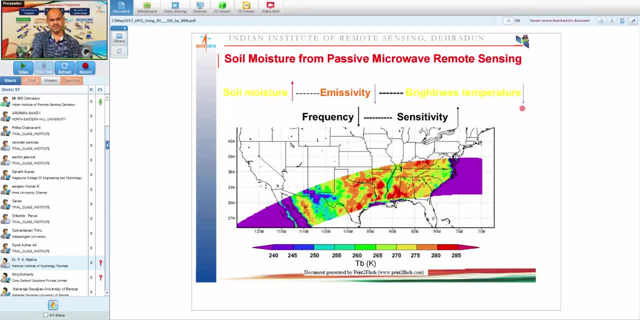 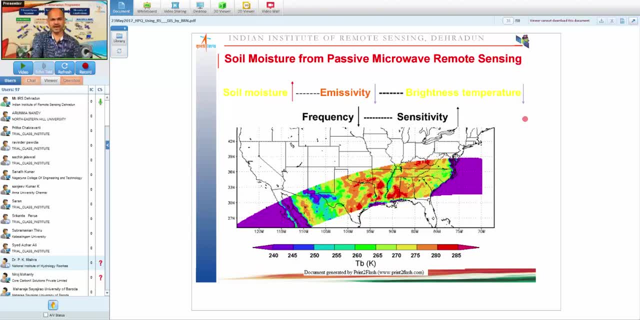 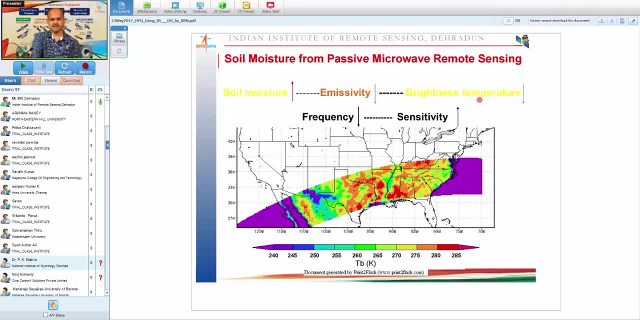 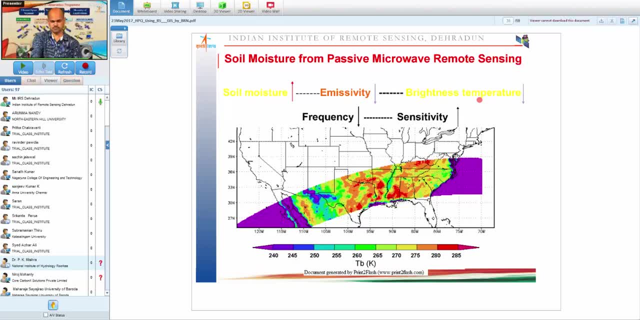 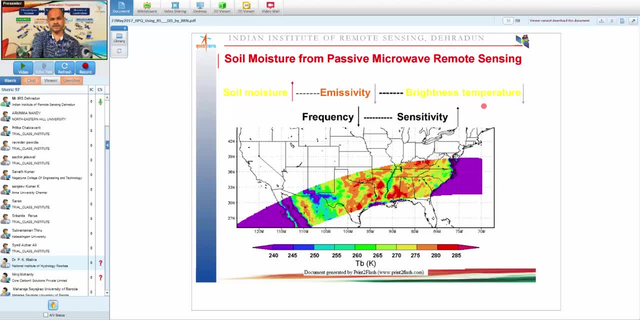 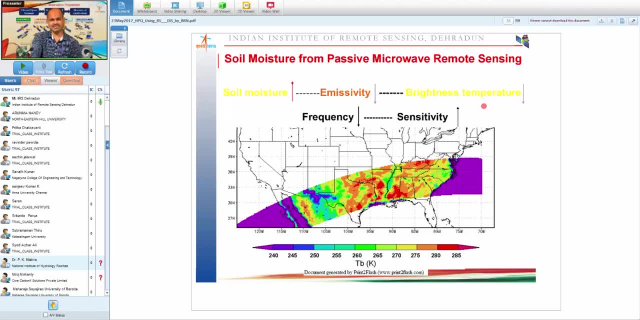 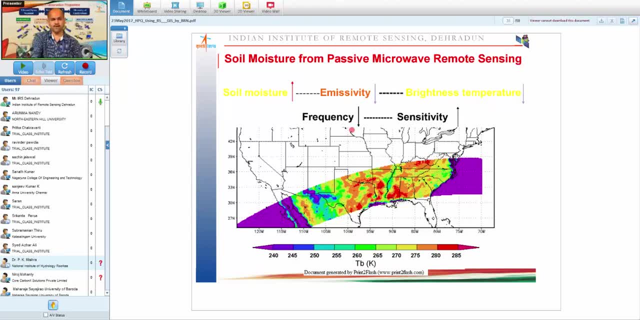 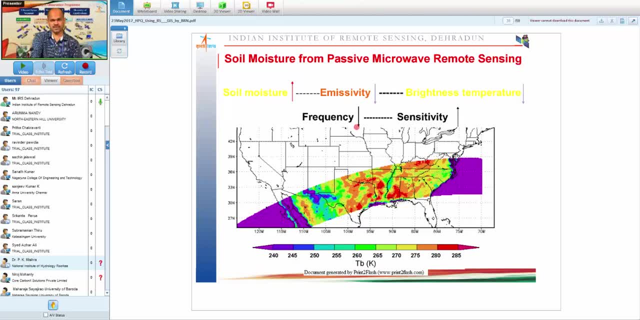 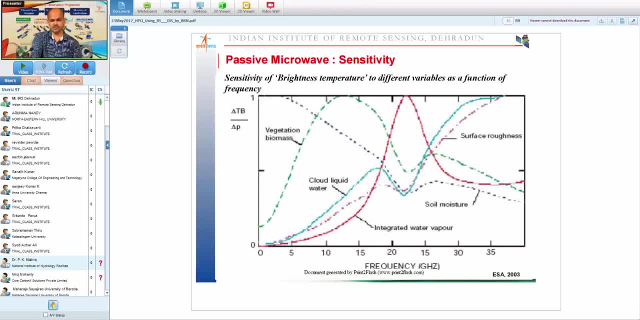 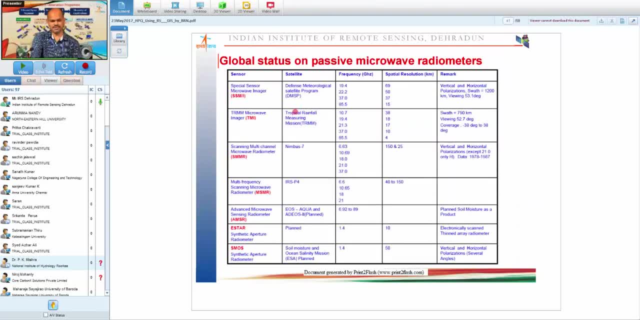 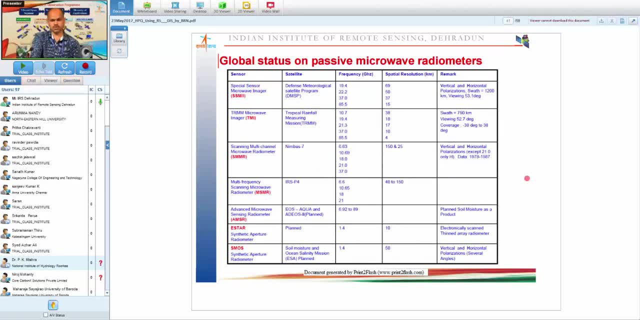 these are the few missions which used to give us passive microwave data. Here in this table I have only listed up to S-MOS. There is a latest one, S-MAP, which is a soil moisture active passive operated by NASA, which is necessarily the L-band. 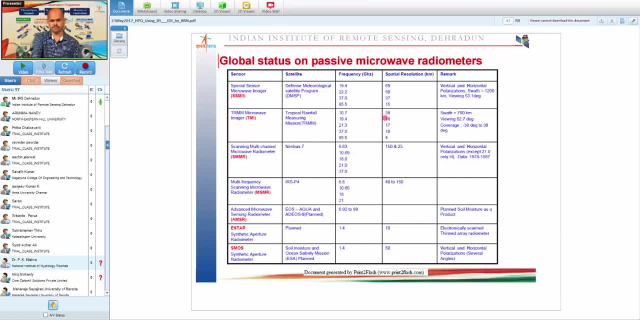 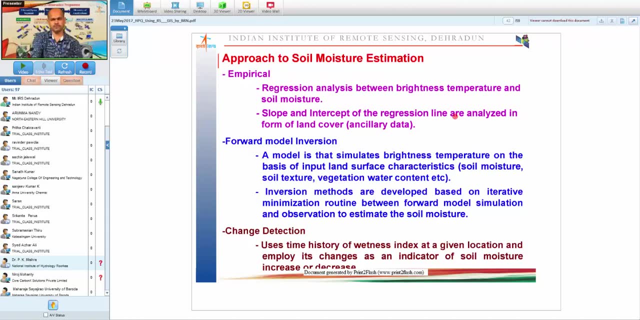 sensor because L-band is the most sensitive band for soil moisture and these are passive microwave sensor having special resolution of the product will have special resolution of in the order of 25 kilometer to 36 kilometer. From these sensors you can retrieve soil moisture using either empirical 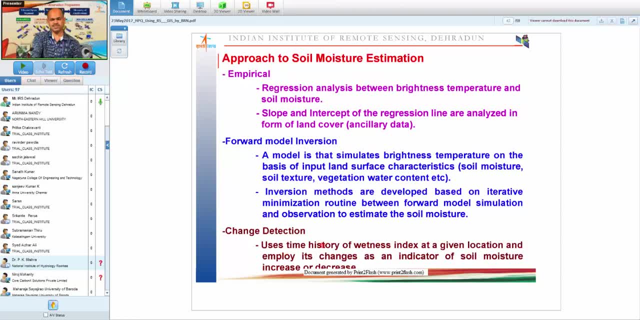 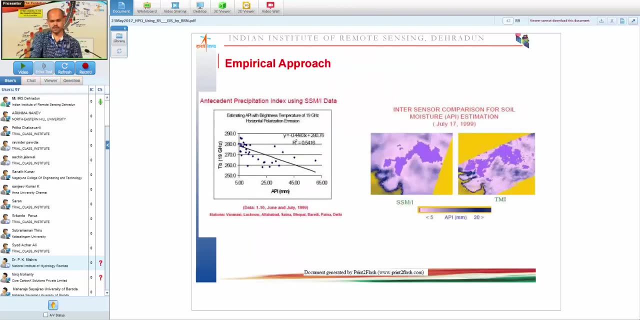 approach, or a forward model inversion approach, or a change detection approach. Empirical approach, as I discussed, you can simply observe the change in brightness temperature and you can correlate the change in brightness temperature with the qualitative status of soil moisture. In forward model inversion, what we do is we observe the brightness temperature in a 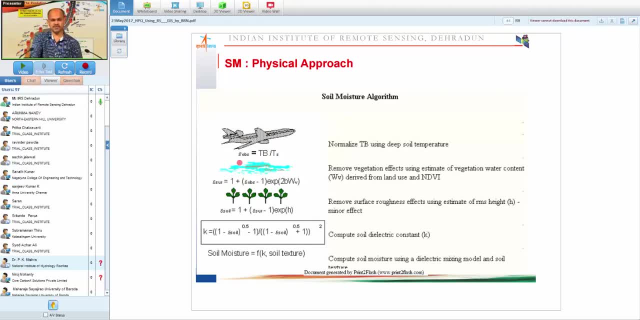 satellite. We try to remove the atmospheric interference in that signal. Then we try to remove the signal which we have received due to vegetation by vegetation correction. Now, whatever signal we have after this purification is the signal is the brightness, temperature, due to moisture available in the soil. Now we say that. 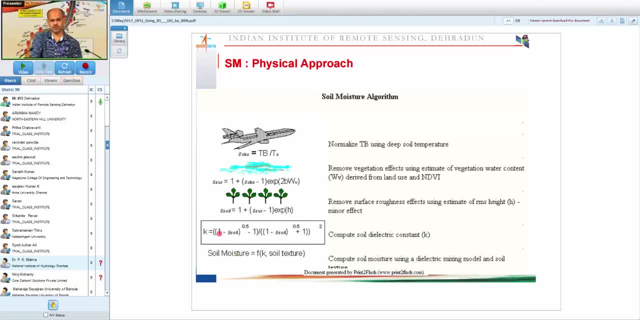 the brightness temperature is a function of dielectric constant and the dielectric constant is a function of, let's say, soil texture and volumetric moisture content in the soil. So you can employ the Inversion algorithm and you can observe soil moisture at some point and you can calibrate this algorithm in iterative. 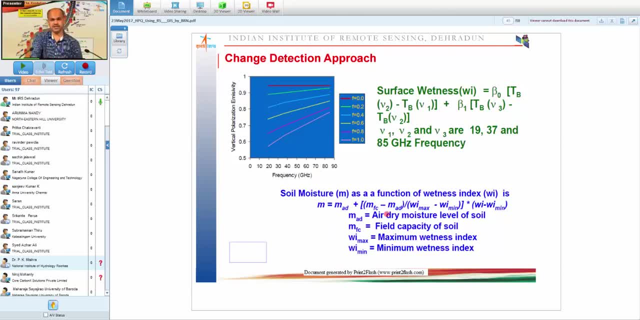 manner Now in change detection. this is the very popular algorithm in case of passive microwave sensor. you can calculatethis is one of thecipheratoms- surface wetness of a pixel using brightness temperature of different channels. This specific algorithm is ingredient of網 joined available of text-resistant soil. So if this 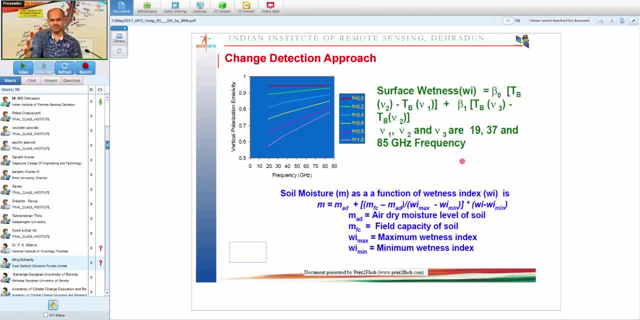 specific algorithm is developed for SSMI sensor where three channels are being used, one, 19 GHz, 36 GHz and 85 GHz. So this is a brightness temperature in channel 2, 36 minus brightness temperature in channel 1, then brightness temperature in channel 3 minus brightness. 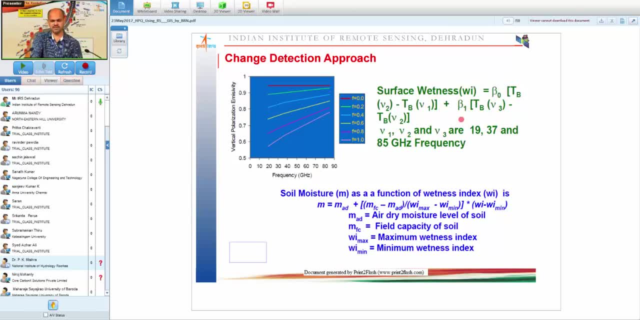 temperature in channel 2.. Now this beta 0 and beta 1 are the constants developed for that specific sensor and that specific algorithm. Now, if I employ this, I can get the surface wetness of all the pixels for all the time. This can give me the quantitative assessment of soil moisture. 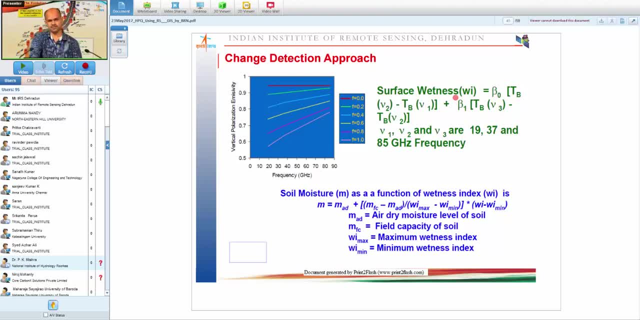 If I want to convert that quantitative assessment of soil moisture into quantitative terms- sorry, qualitative assessment into quantitative terms- I need some observations So you can see here the soil moisture of a specific pixel for a specific time can be calculated if I know soil. 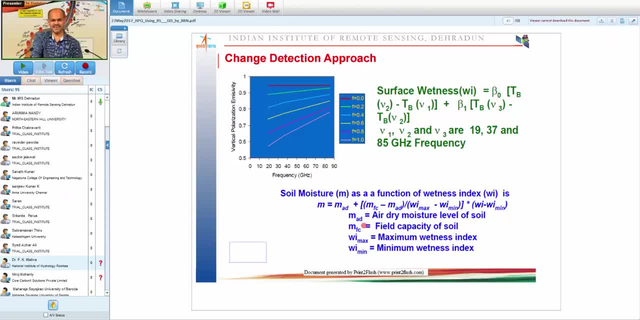 moisture if the soil is air dry, and then I will add difference in soil moisture when the soil is at field capacity minus soil at air dry. divide it with the wetness index when soil is at field capacity minus wetness index, or when the soil is dry, and then I will multiply it with the difference in today's wetness. 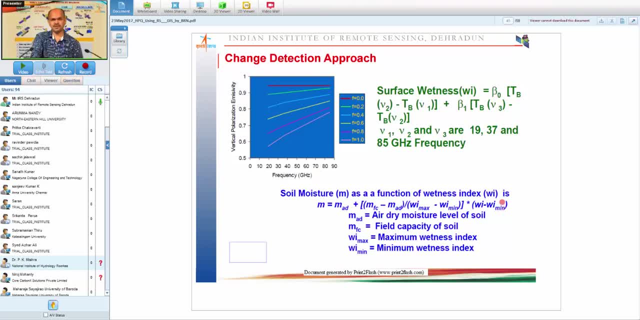 index and the minimum wetness index. So I am just calculating difference in the datum wetness index and today's wetness index and the moisture between those two values, and then I am adding it in the air dry soil moisture. So this algorithm will give you quantitative assessment of soil. 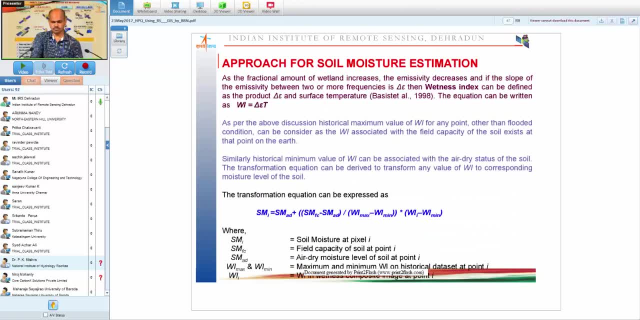 over entire area for all the time periods We will skip. The limitation will of course be: you need robust observations to generate these relations, But if you can do extensive field observations with time, this can be done and operationally this has been done, So you can. 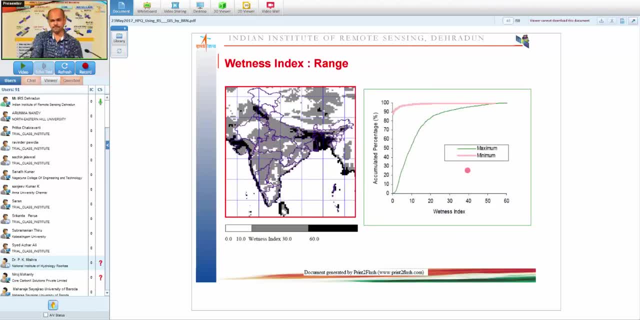 do a lot of analysis and you can do a lot of calculations. So you can do a lot of calculations. So you can, for around last 25 years where you can see the wetness index, you can correlate with the antecedent. 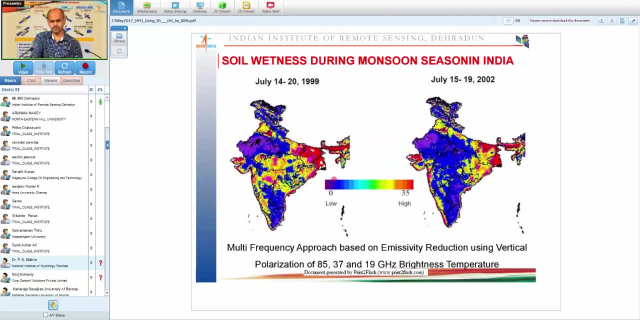 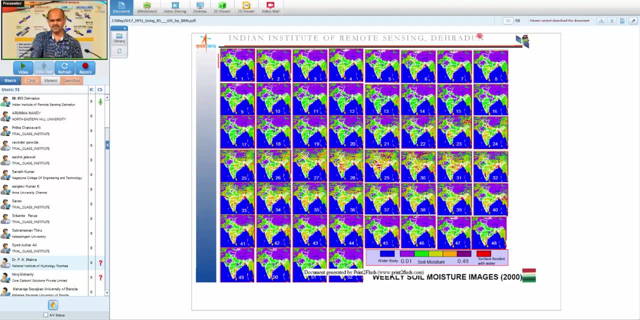 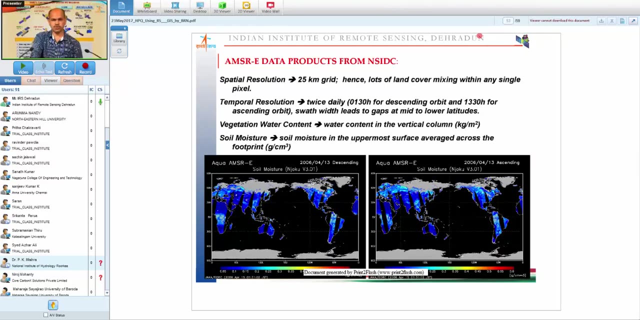 moisture condition which is a rainfall in that area. Here you can see the wetness index you can represent for the different time periods. Now from wetness index, soil moisture for entire country or entire continent can be calculated. Now, as Dr Praveen told you, AMSRE and AMSRE2 has number of 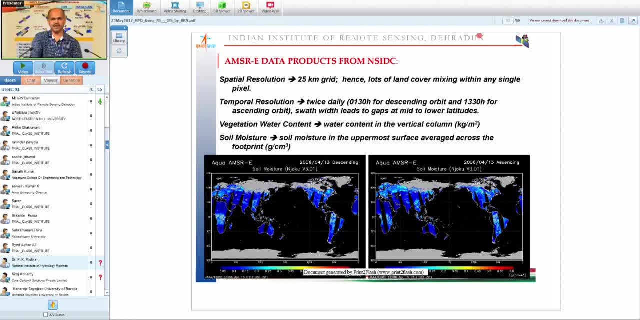 passive microwave channels. using those data, either using by change detection or using forward model inversion algorithm, soil moisture can be retrieved and there are products freely available in which C band and X band passive microwave brightness temperatures are used and the long frequency, like 89- 85 gigahertz frequency, is used for calculating surface. 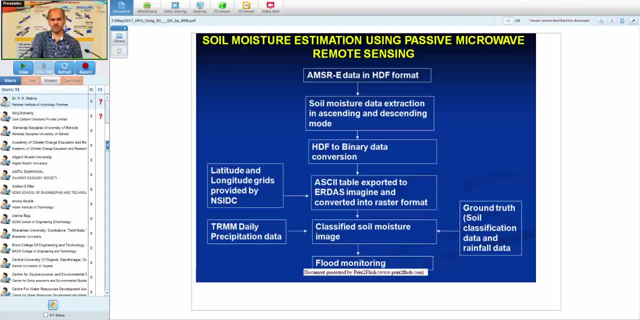 temperature and then these values are put in inversion algorithms to calculate soil moisture. so these products are available. you you have to do some pre-processing of those products where you have to merge them. gap filling you have to do and you can get these products on daily or weekly. 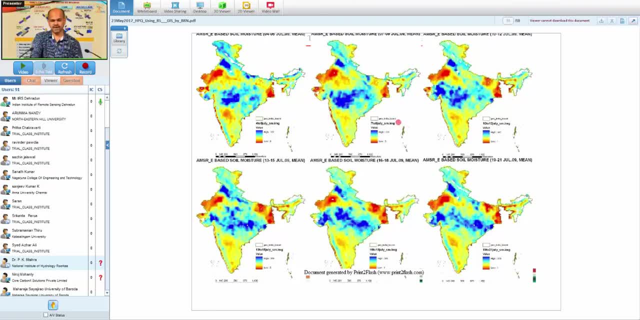 time scale, which I'm showing here for a fortnightly or weekly time scale, you can observe the status of soil moisture for entire country or entire continent. this is a case of 2009 where we were facing drought, like situation in early monsoon. you can see here: the blue part indicates the high 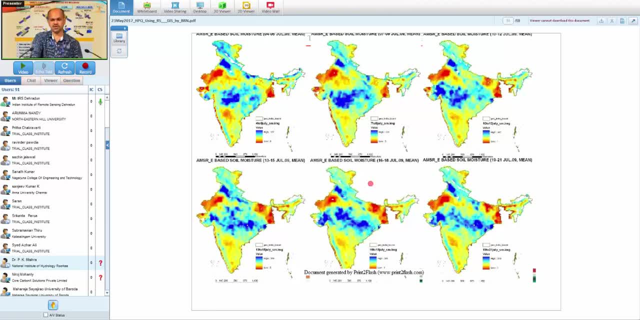 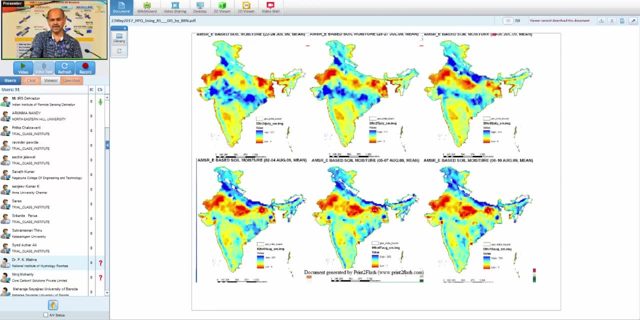 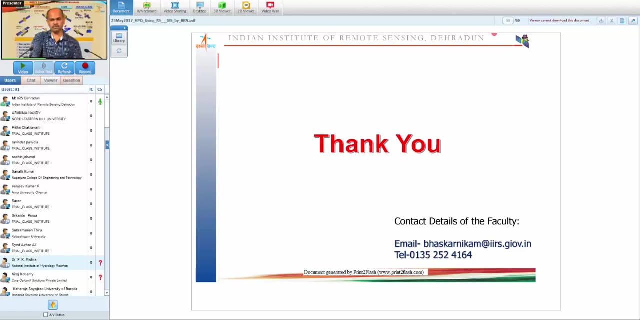 soil moisture condition, whereas the red part indicates the low soil moisture condition and this specific soil moisture progression indicates the progress of monsoon. I can correlate this with progress of monsoon. so, using this product, if, let's say, you want to use this product in your hydrological modeling, because soil moisture is an essential input. 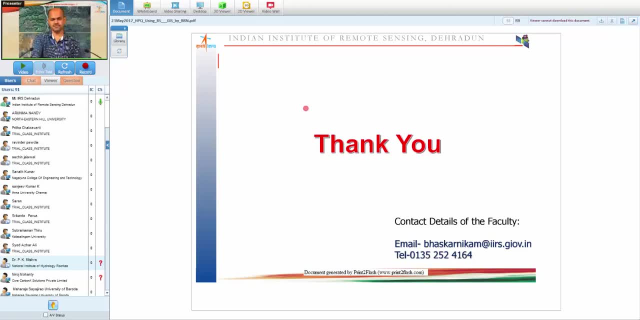 in hydrological modeling so you can use this product. if you don't want to retrieve these products, the freely available product from AMSRE, AMSRE2, SMAP and SMOS can be used, can be either forced in your hydrological model or can be, let's say, assimilated in a hydrological model to improve. 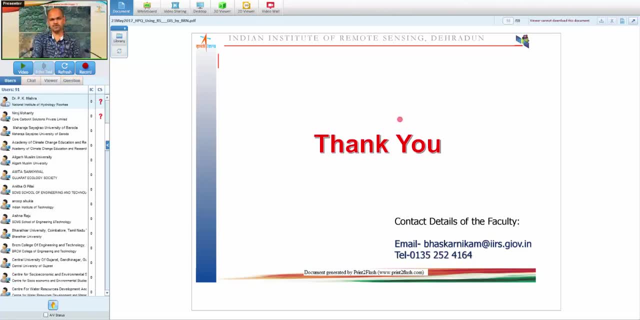 the accuracy of that model. now, today we have not touched upon one topic, which is a terrestrial water storage, which we will touch in coming lecture. so we calculate terrestrial water storage. you can calculate it using volume. and that's it for today, for today's lecture. thank you for watching and we will see you next week with a new video. 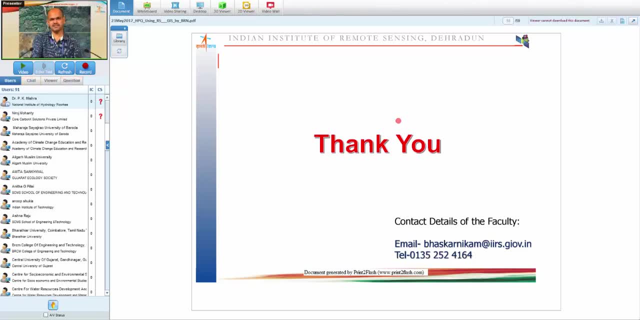 limb balance approach. you calculate all other parameters and the Delta in those parameters is a terrestrial water storage. there is an alternate approach wherein we use remote sensing data of a gravity satellite to calculate get a terrestrial water storage. as you know, the gravity field will change if the 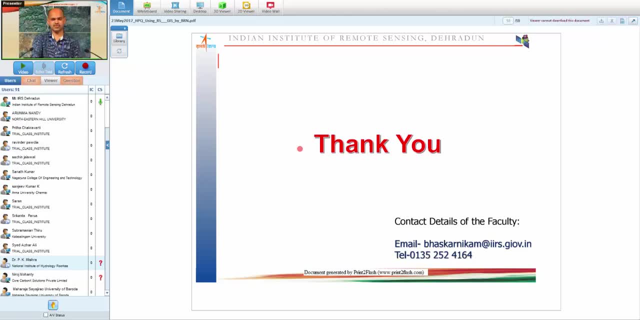 density of object or the surface is changing and the density of surface or the mass of surface changes with a change in water storage, either a surface water storage or soil moisture storage. so that change, that that minute change, is observed by twin satellite, which we call grace satellite, and that is. 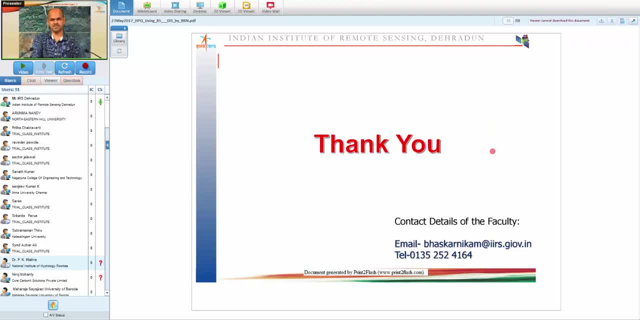 converted into terrestrial change in delta TWS, change in terrestrial water storage, which is also very important parameter for your soil moisture, as well as groundwater. status of the assessment, which we will discuss in coming lectures. so this concludes my presentation on hydrological parameter estimation. now, if time permits, we can take some.